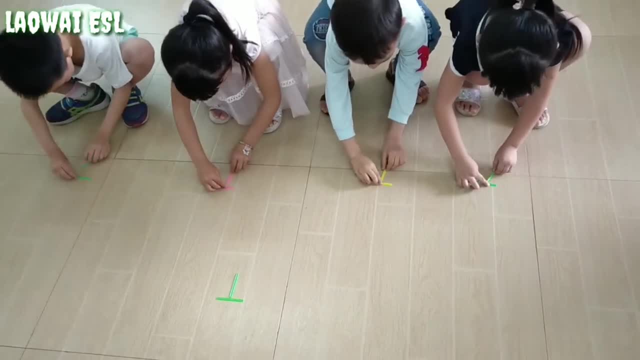 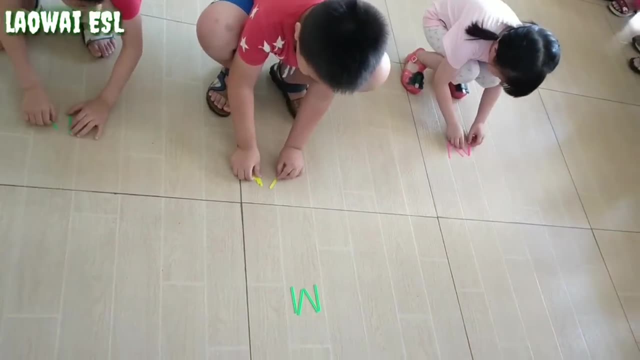 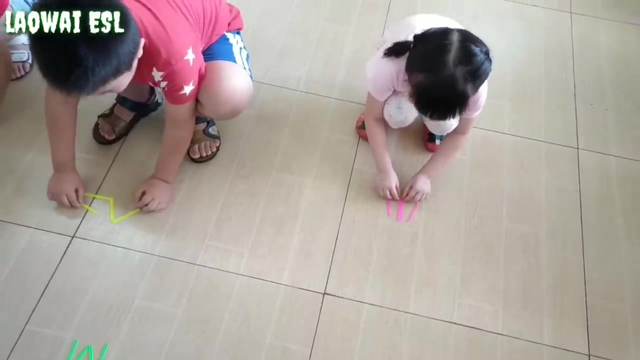 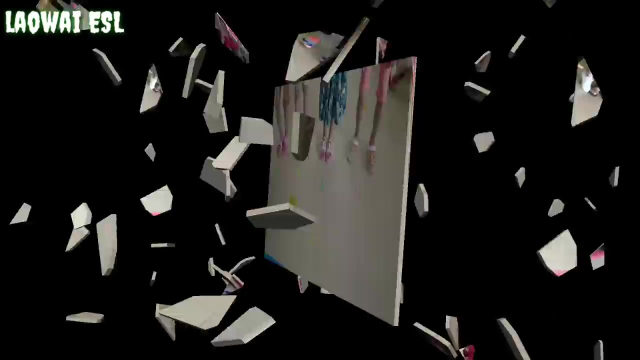 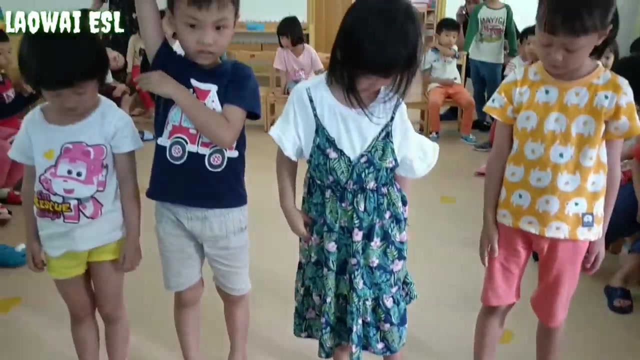 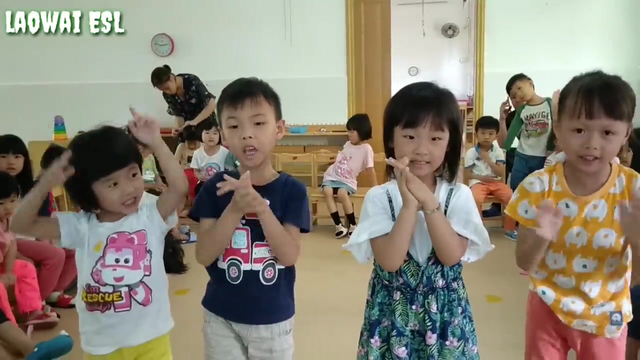 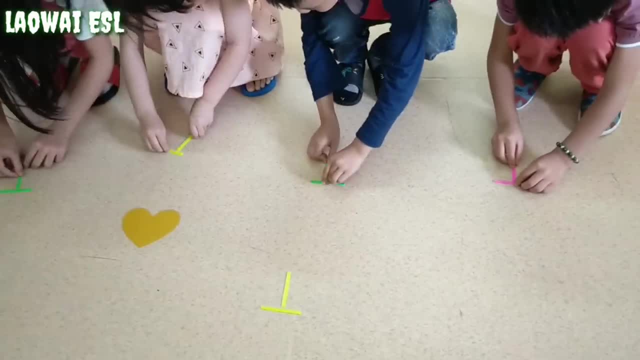 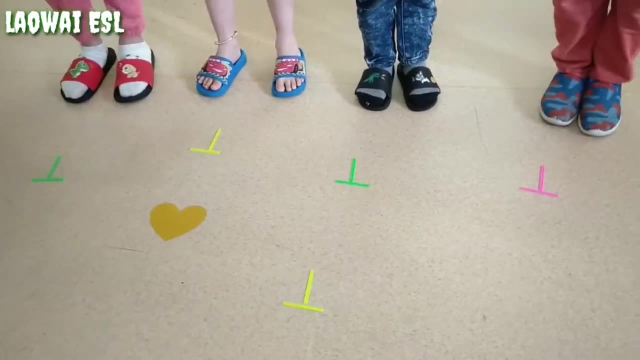 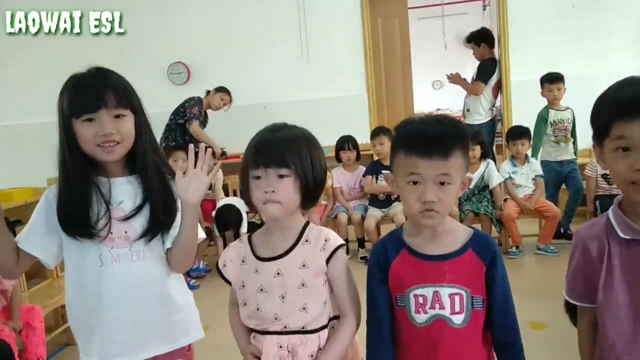 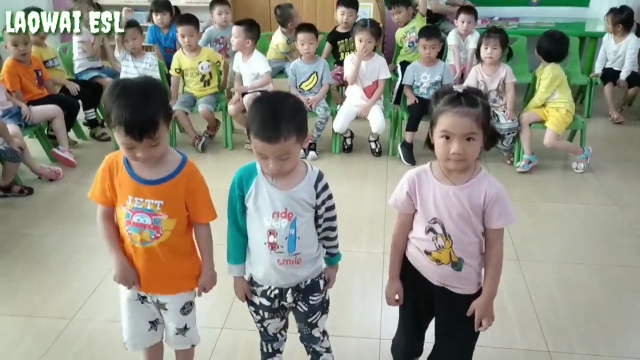 Let's go, let's go. let's go. Create letter T. Very good, Well done. All right, Everyone put your hands up and say T, T, D, T, Well done. Come back and sit down. One, two, three, Let's go, let's go, let's. 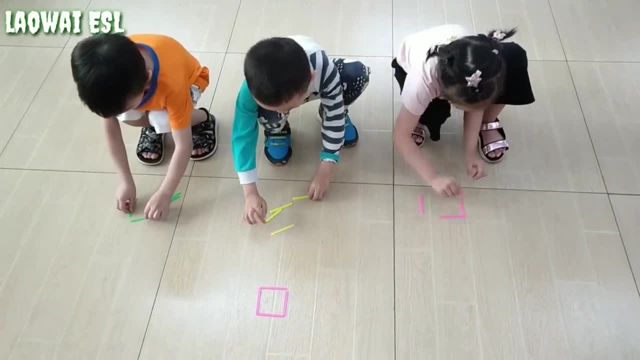 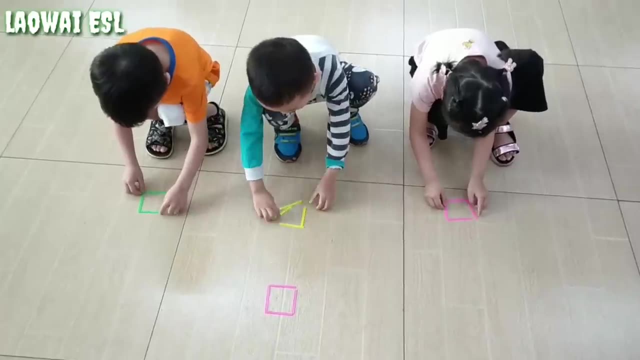 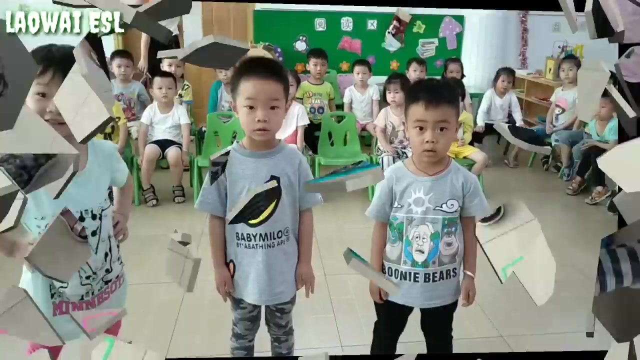 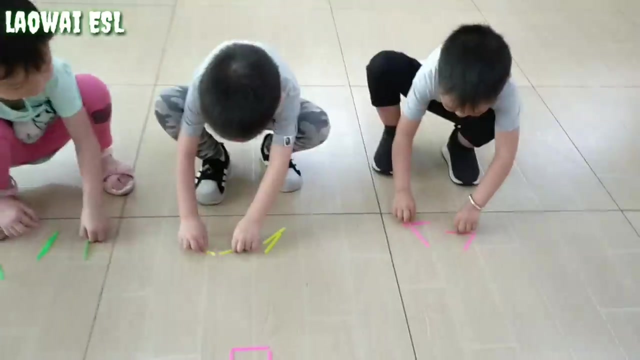 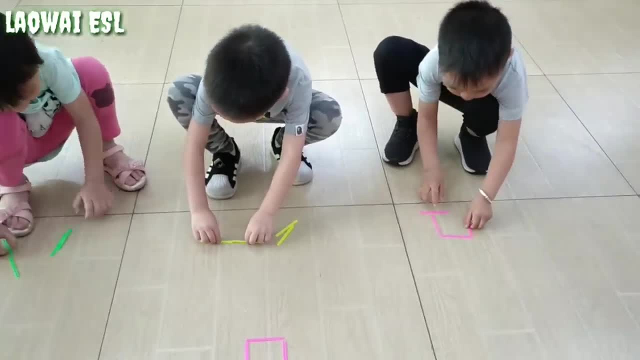 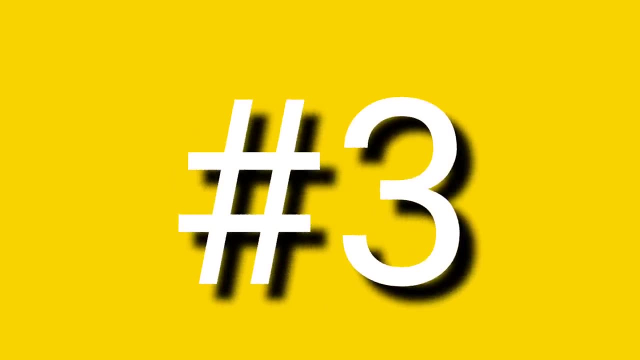 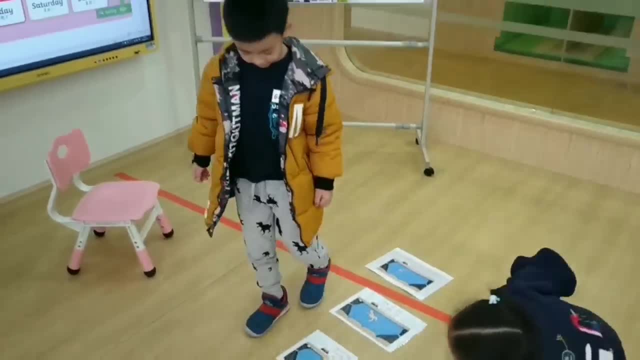 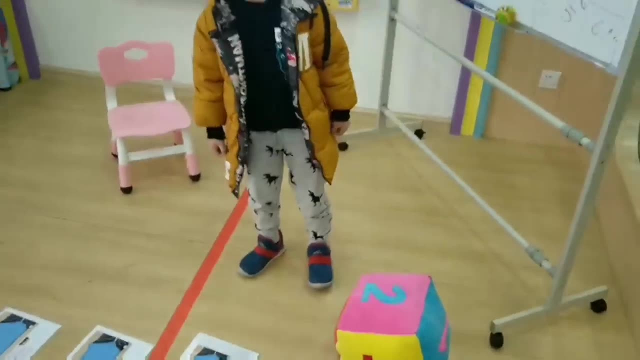 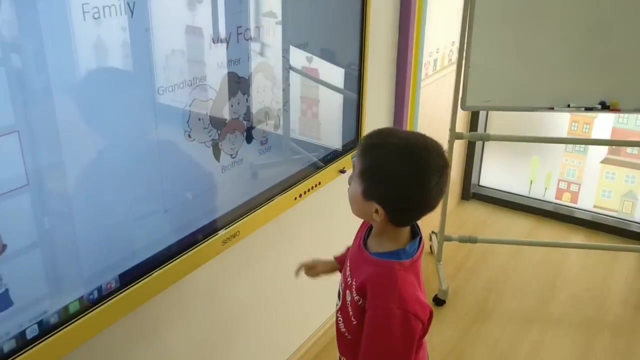 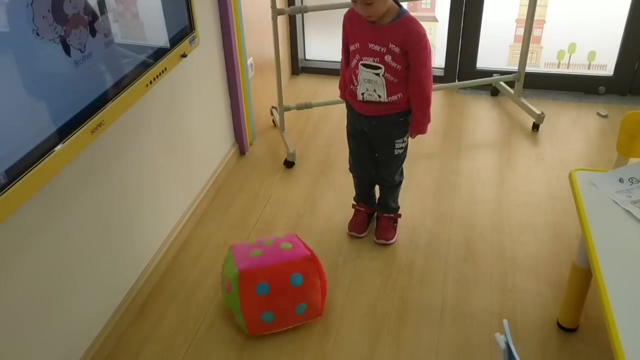 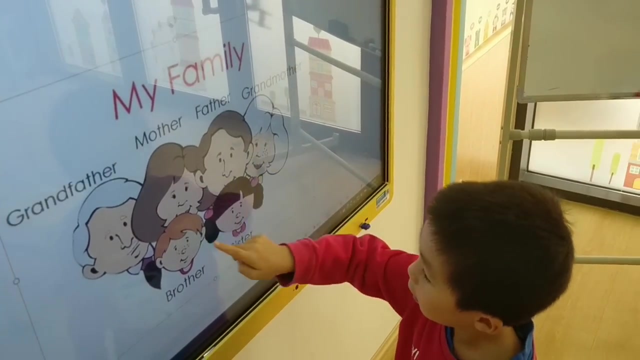 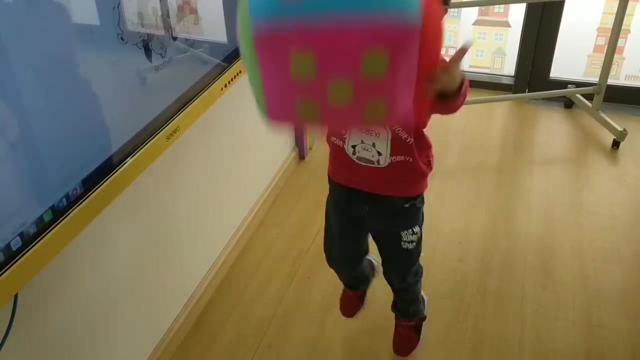 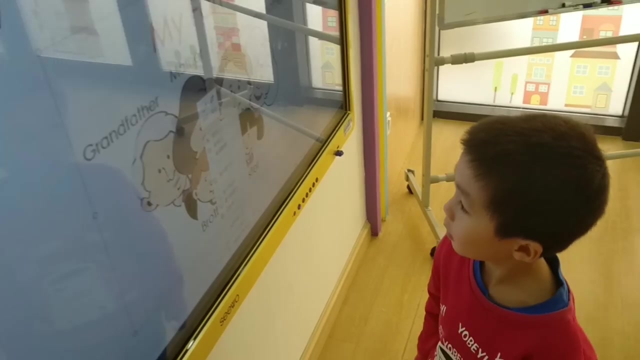 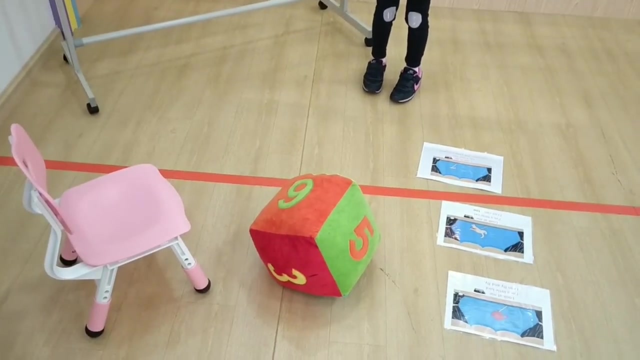 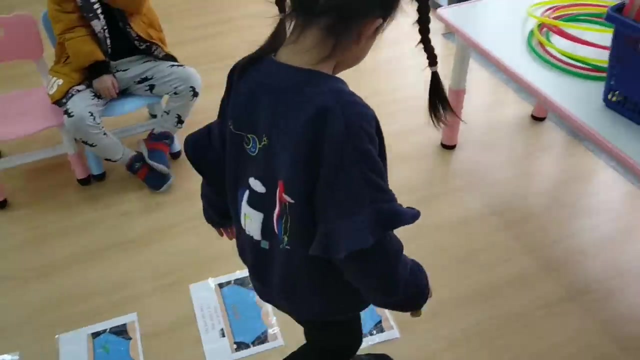 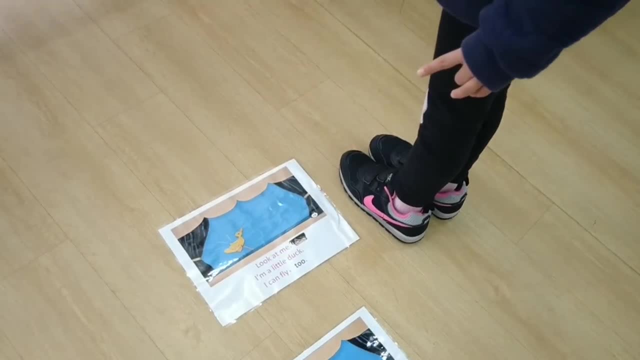 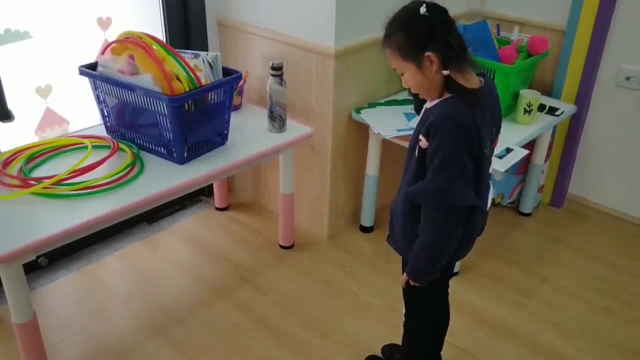 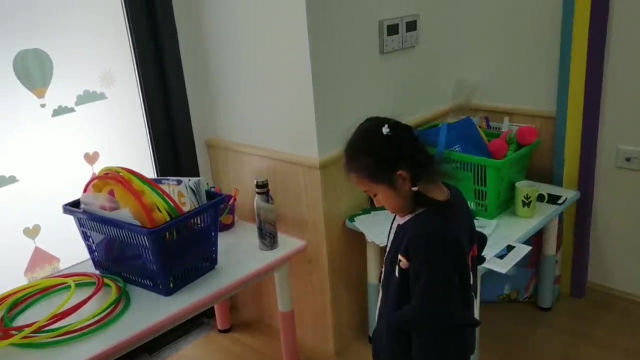 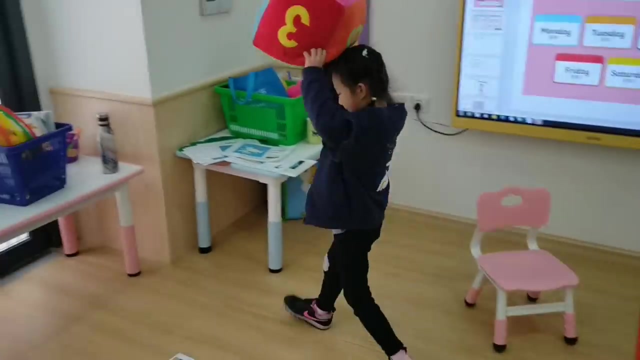 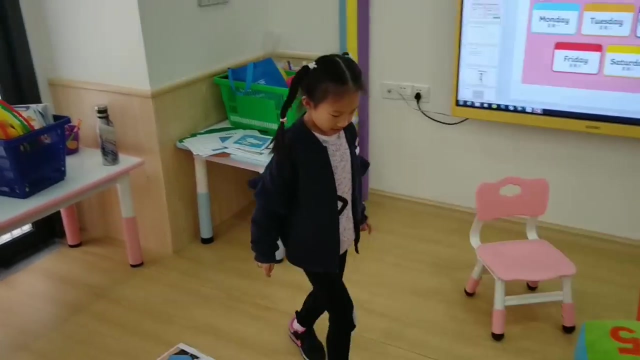 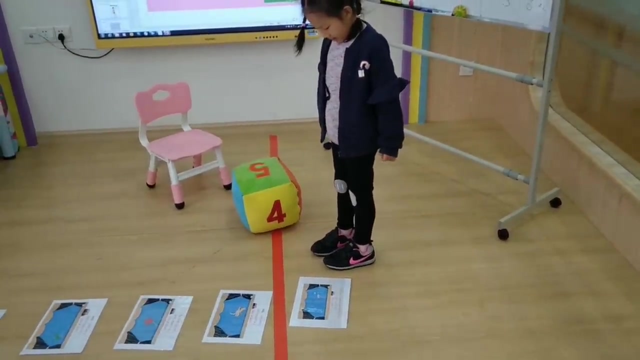 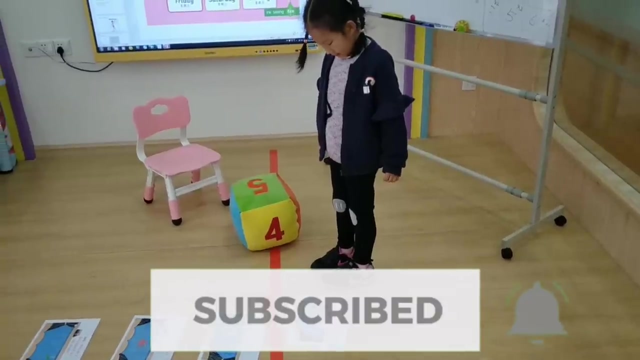 look at me, I can fly. well done, let's continue. number five: number five: number five: one, two, three, four, five. All right, Look at me, And a little fish And a green and green and green, Wonderful. 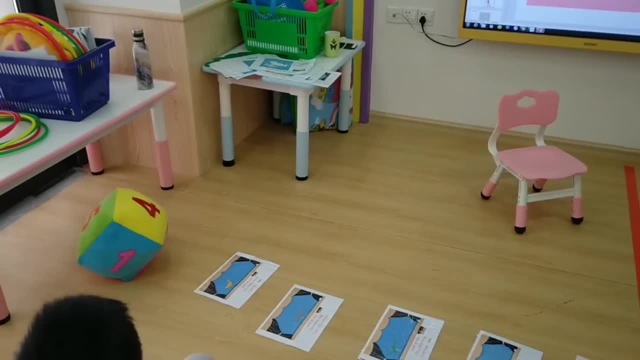 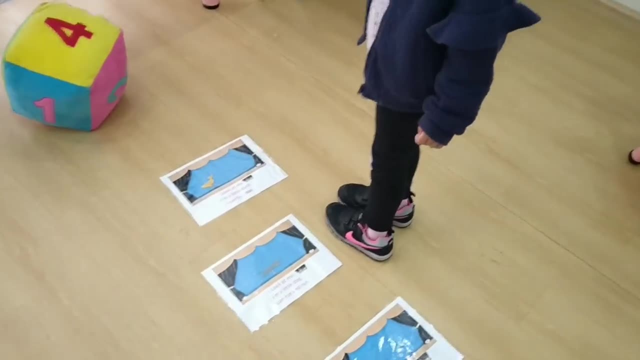 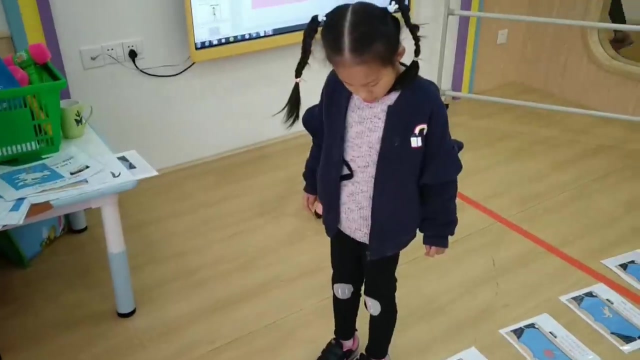 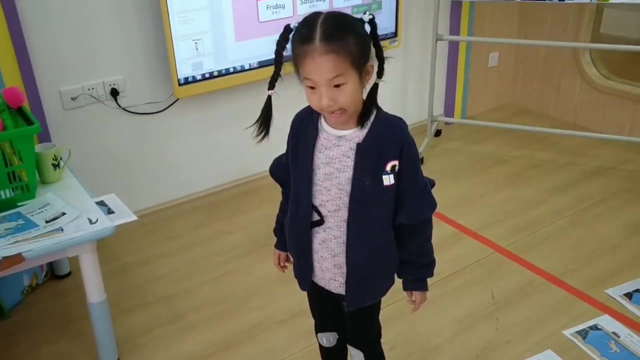 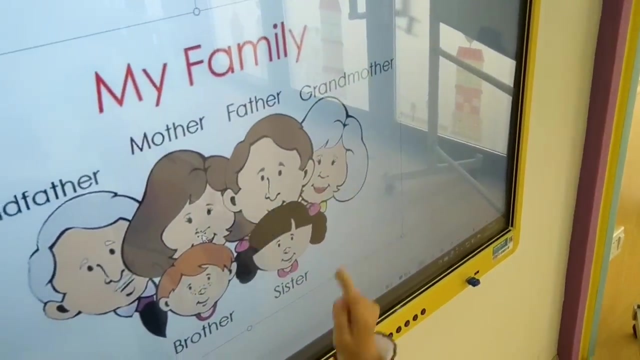 Come on: One, two, three, four, five. Come on, Have a dream, Look at a little dog And run and run. I can run and run. I can run Five. One, two, three, four, five. 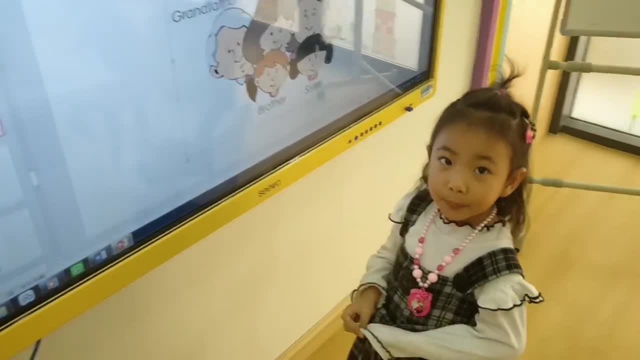 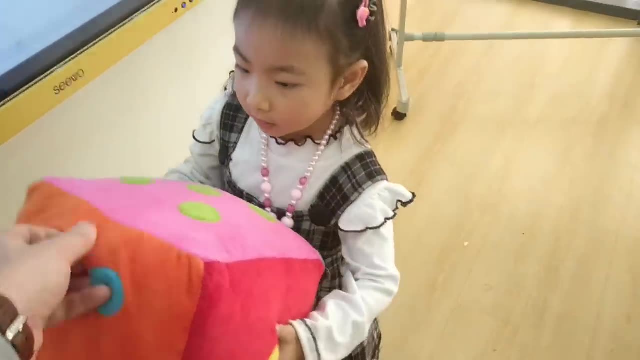 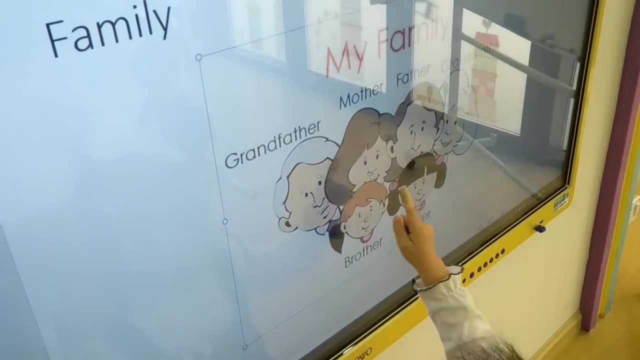 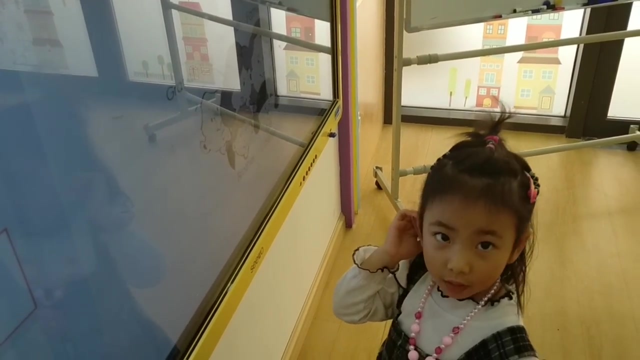 Who is he? He is my baby. He is my brother. He is my brother. Let's do that again. Come on, Shake it. One, two, three. Who is he? He is my brother. Very good, What number is this? 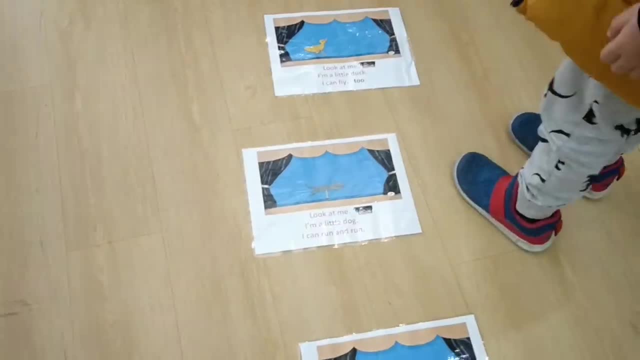 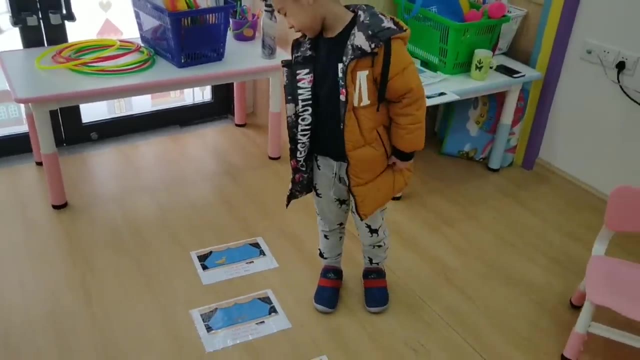 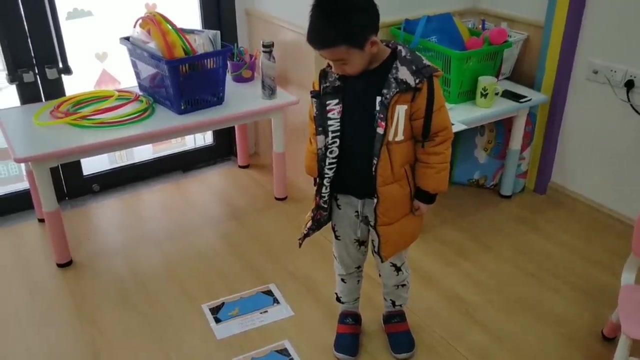 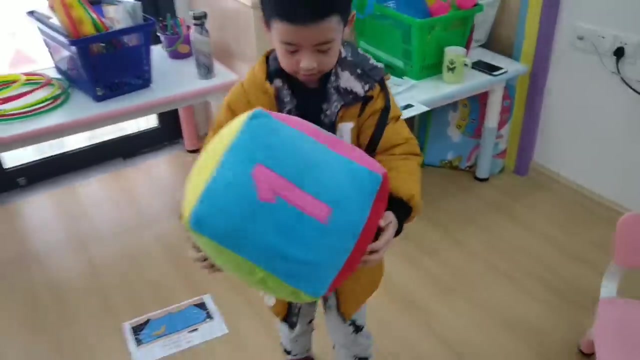 One. All right, Look at here Here. Look, Everyone can see. Oh, I can run and run. Look at me, Look at me, I can run and run, and run, I can run and run. Okay, let's continue. 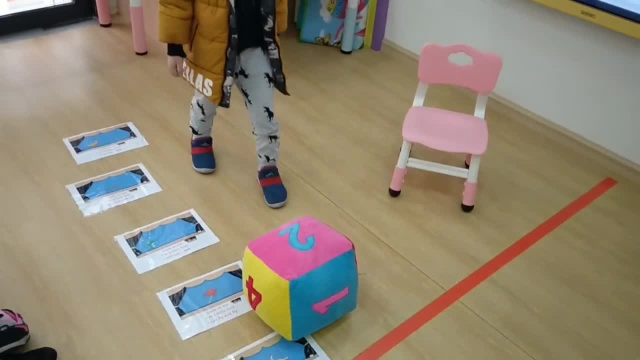 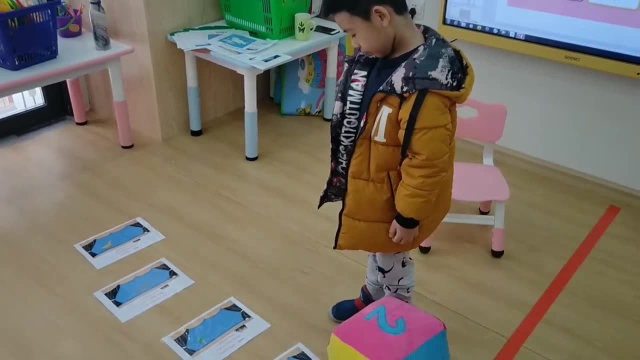 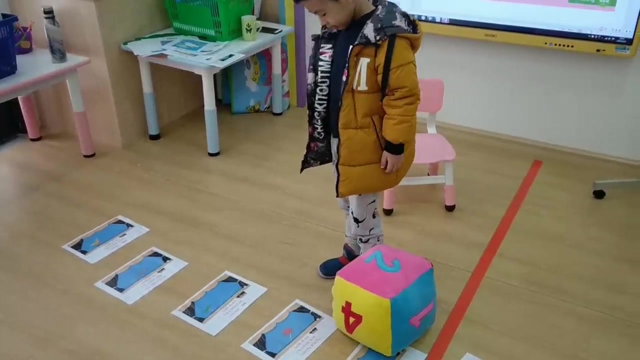 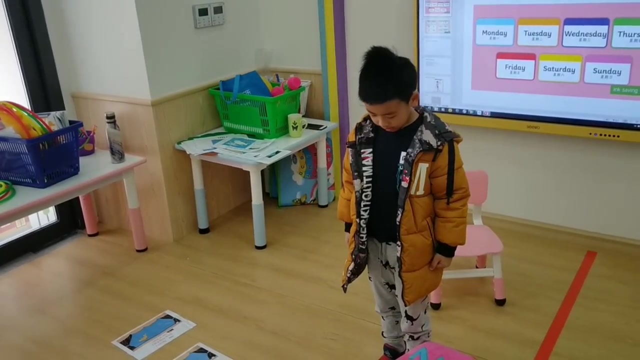 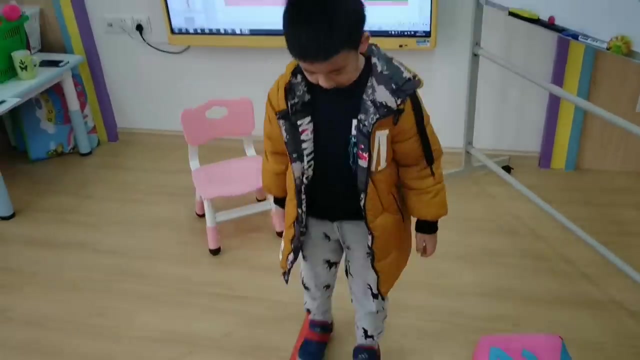 One, two. look at me. Look can run and run. I can run and run. The others will join us. No one can beat me. I can fly and fly. I can fly and fly. Let's continue. One, two. 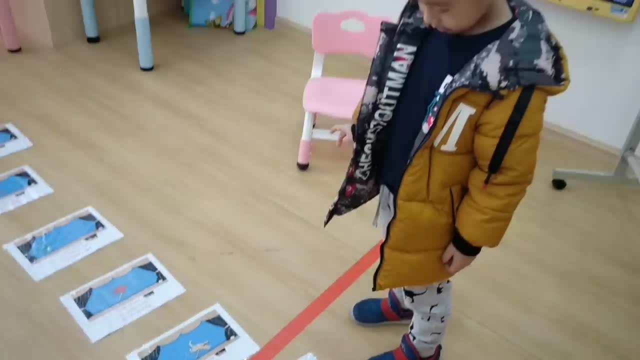 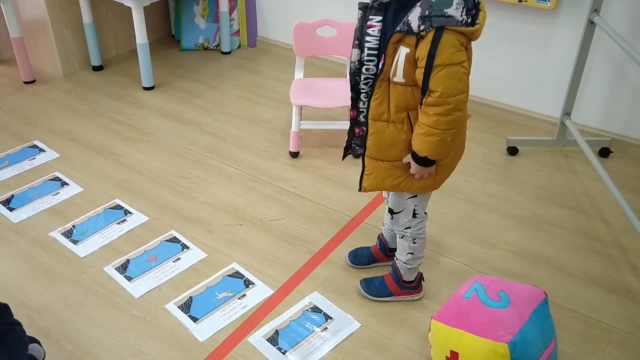 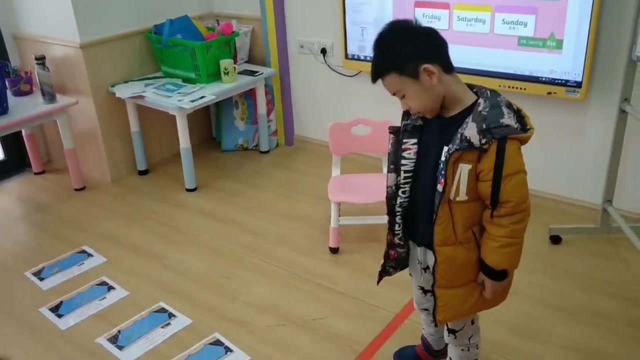 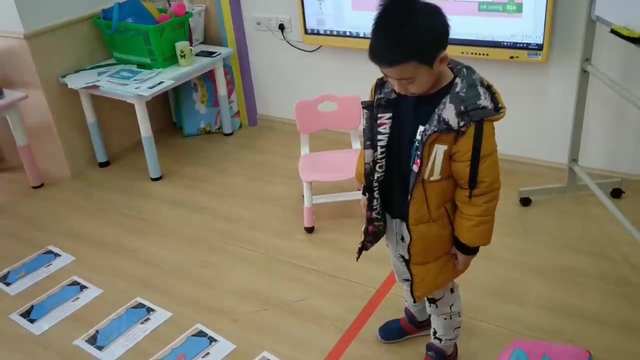 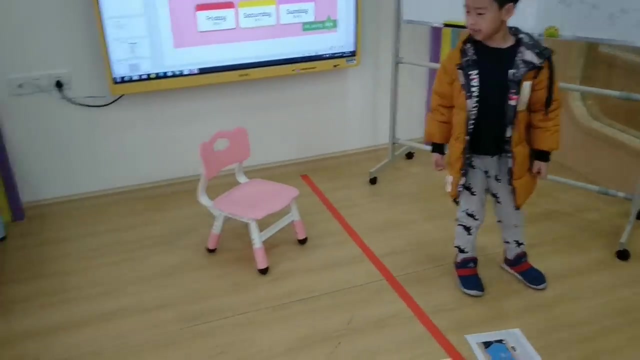 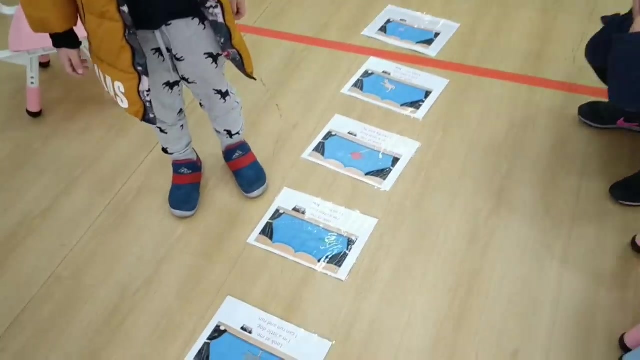 Mm-hmm, Look at me, I am a little fish. I am a little fish, I can swim and swim, and swim. Very good, One more time, One, two, three. Come on, Look at me, I can swim. 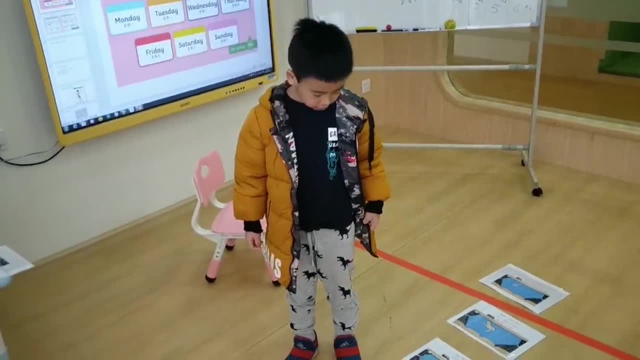 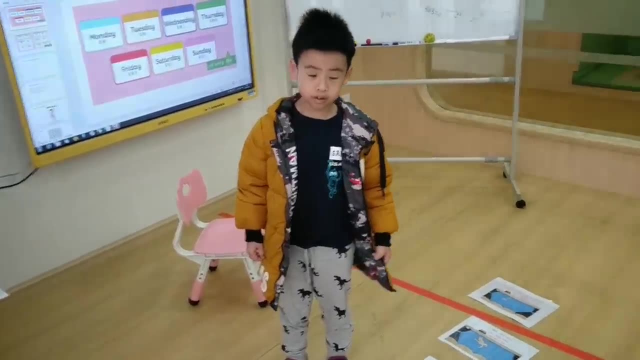 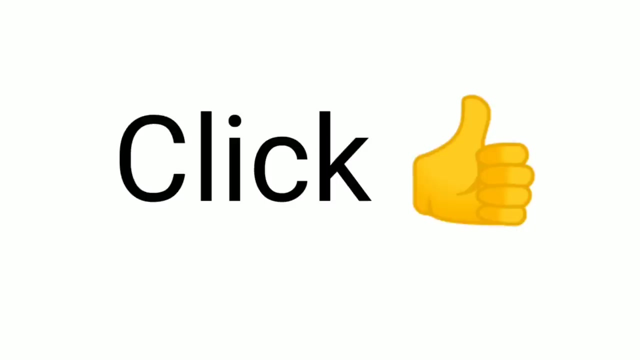 I am a little frog. I am a little frog, I can hop. I can hop too. Okay, good job, Come back and sit down. Good job, One, two, three, four, Sit down, Keep going, Stay in position. 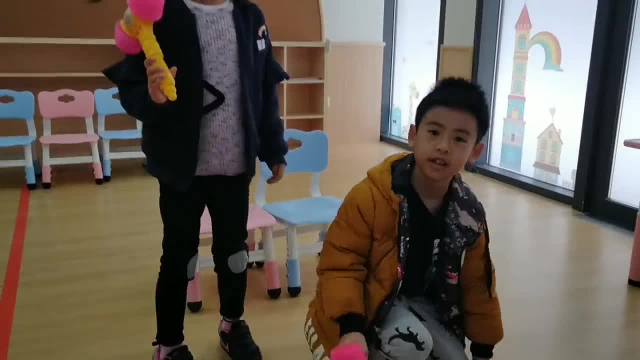 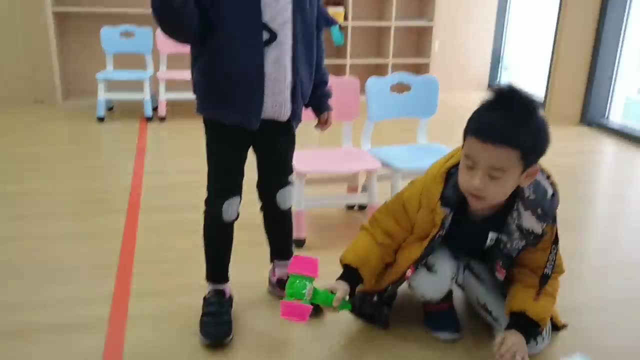 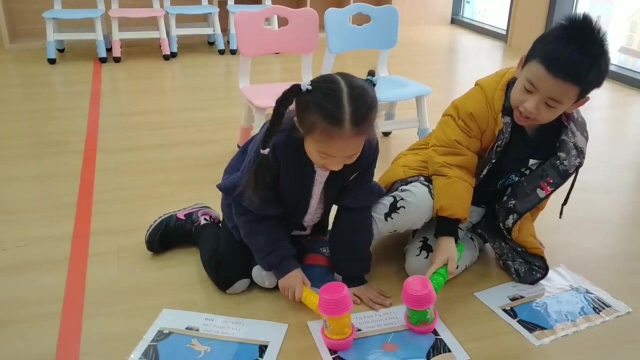 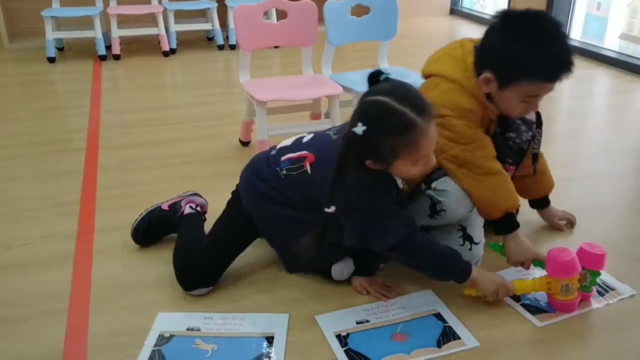 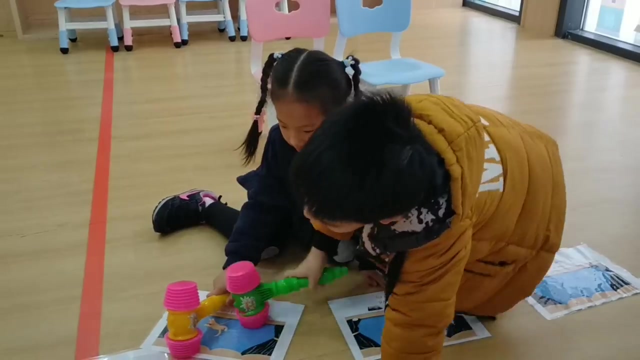 Very good, Welcome back everyone to the還有. I amIsn't a special guest here. This is just the first time he is here. This is the first time he is here: Run, Swim Hop, Fly Run. Swim Hop, Fly Run, Fly Run. 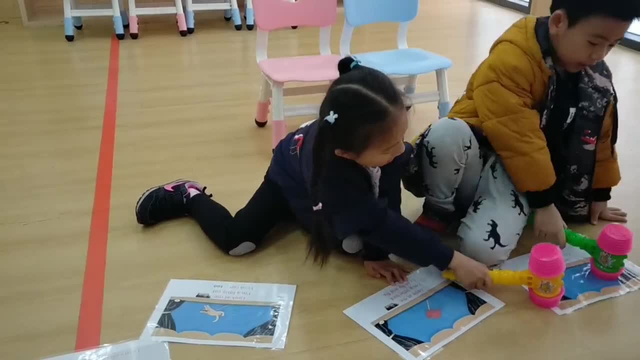 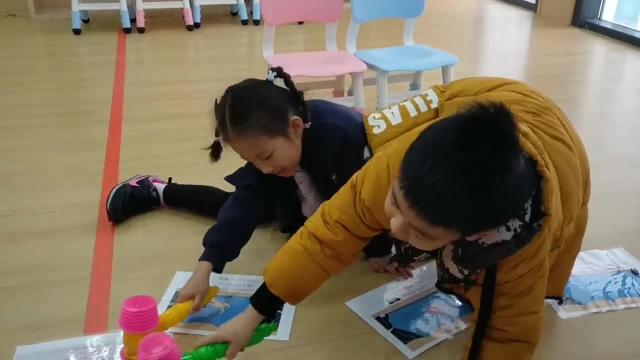 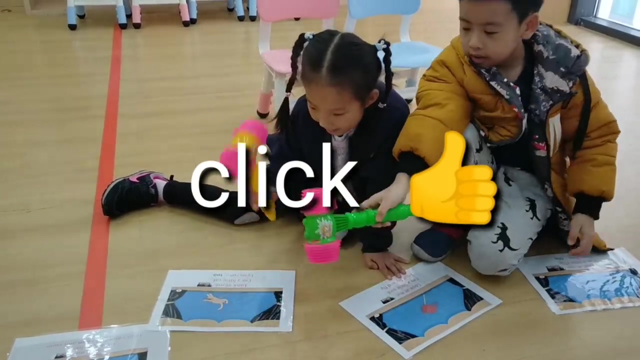 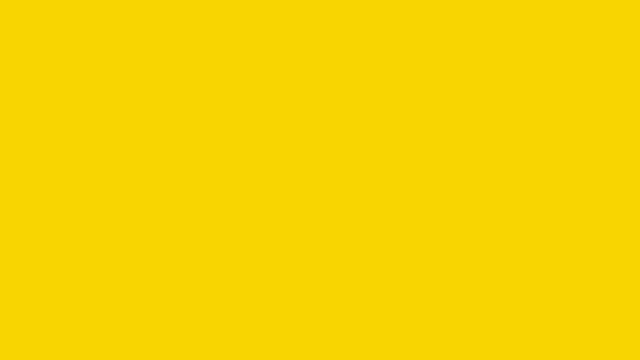 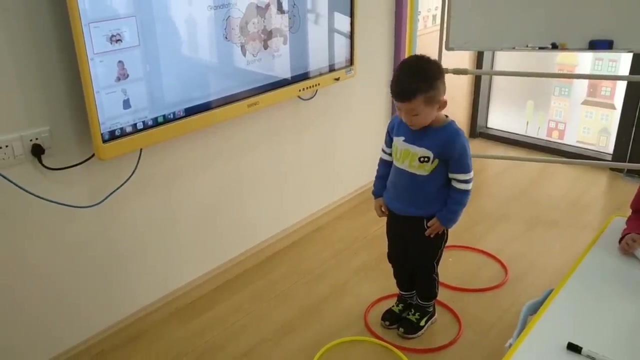 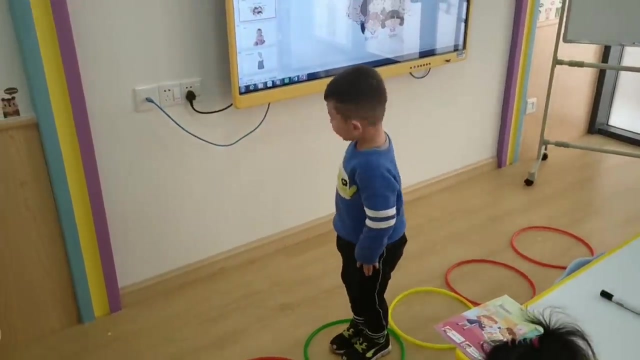 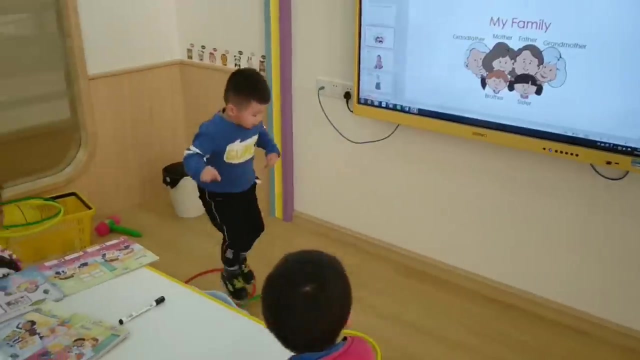 Run, Hop, Fly, Swim, Fly, Swim, Run, Hop, Let's go. He is a Minecraft robot. She is my mother, She is my father, She is my grandmother, She is my brother. Wonderful, She is my sister. 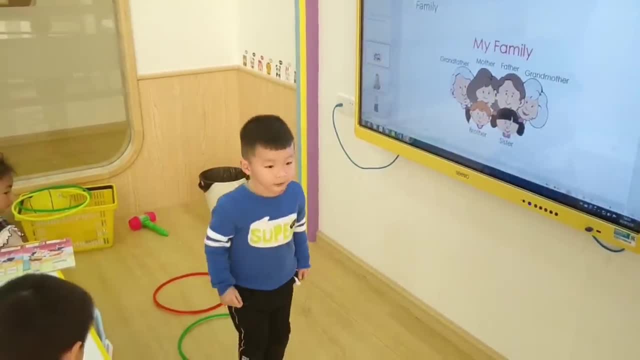 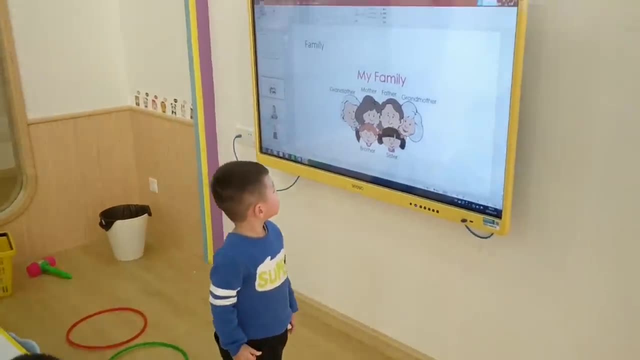 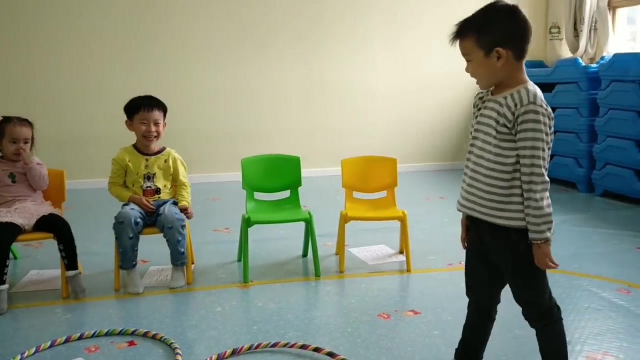 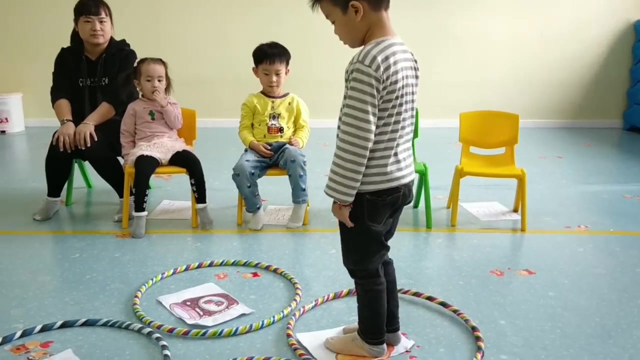 Okay, Okay, She is my grandmother, She is my mother. Well done, She is my father. Very good, Come back, please. I didn't say anything Now. juice- What should you say? Juice, Very good, Jam. 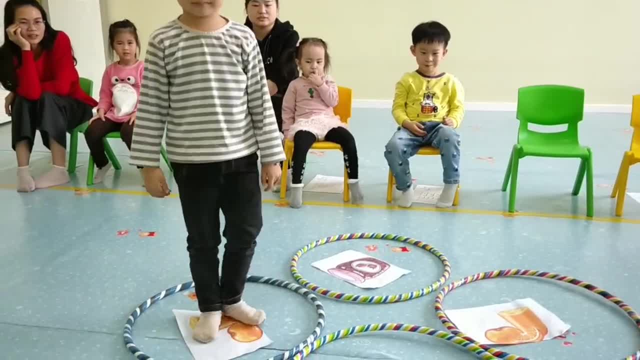 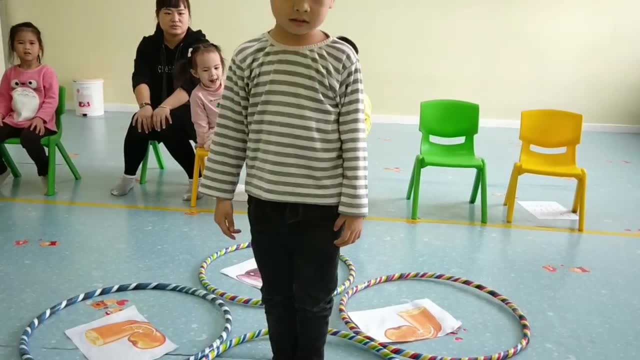 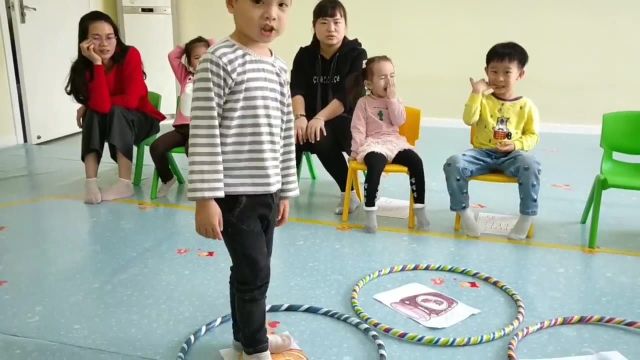 Jam. Wonderful Juice, Juice, Jam, Jam, Juice, Juice, Juice, Juice, Juice. It's not juice, man, Juice, It's not juice. Juice, Juice, Juice, Juice, Ah, Juice, Ah Jam. 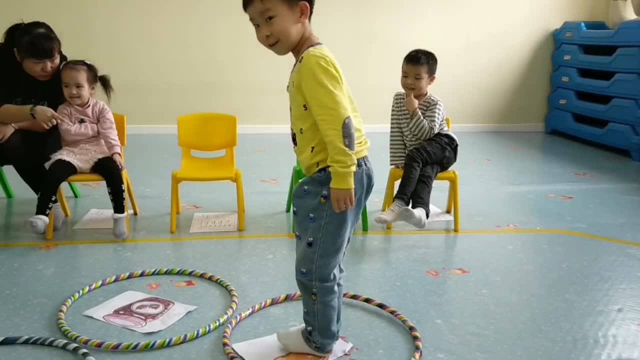 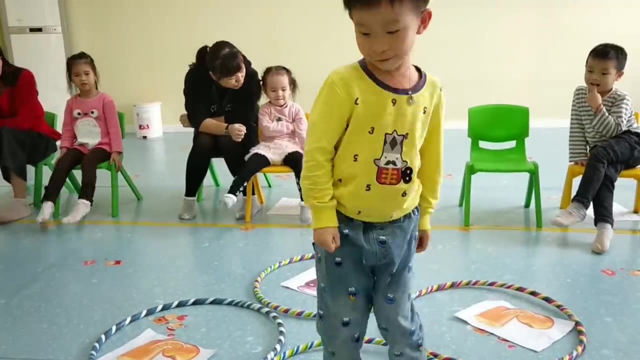 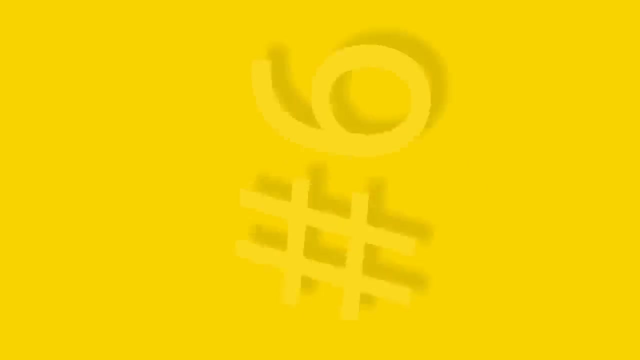 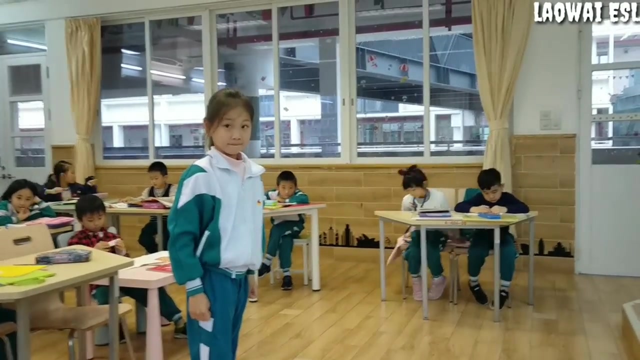 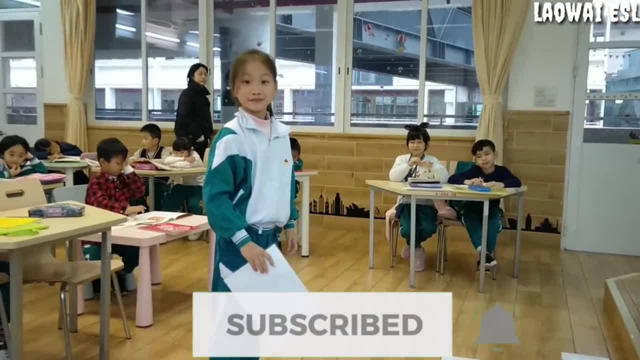 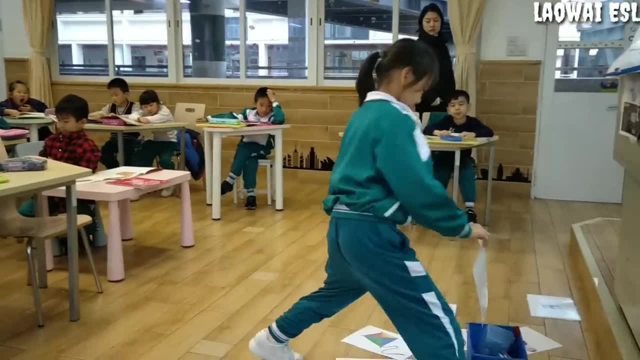 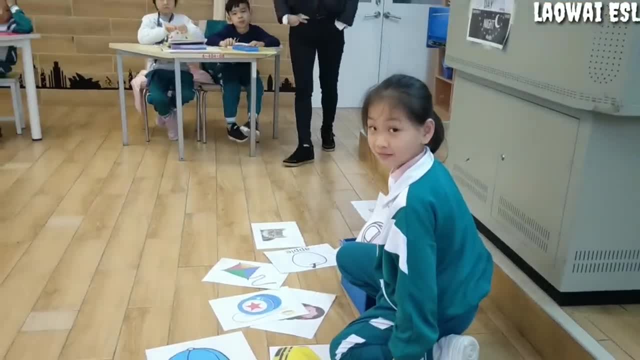 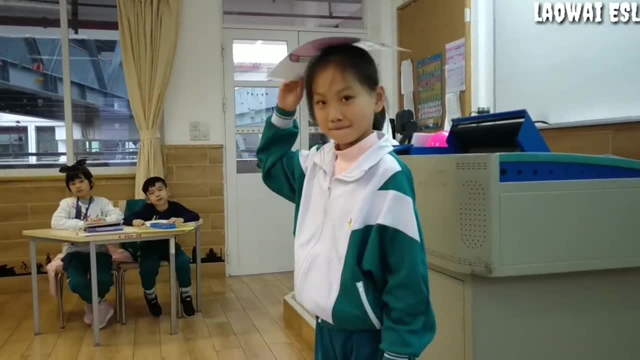 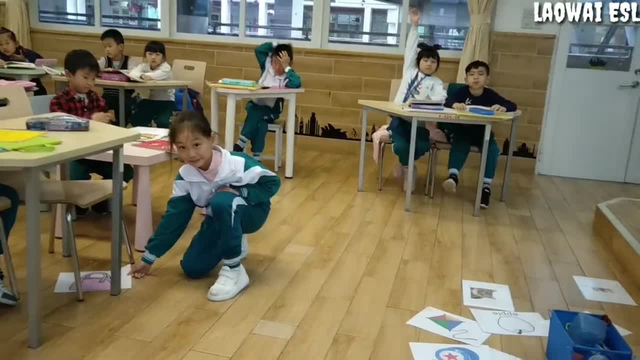 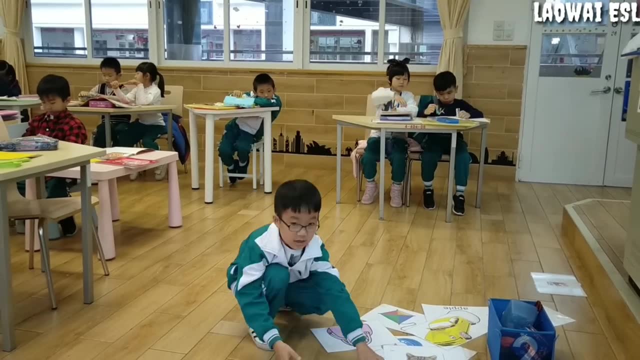 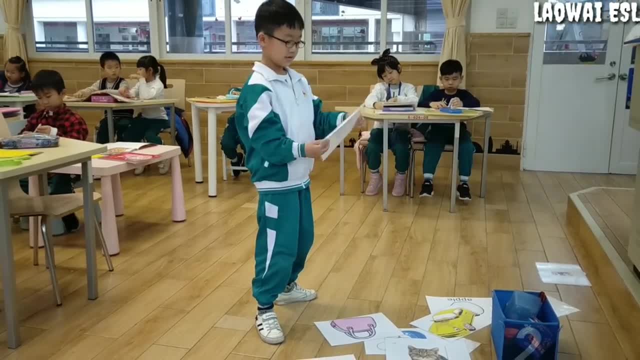 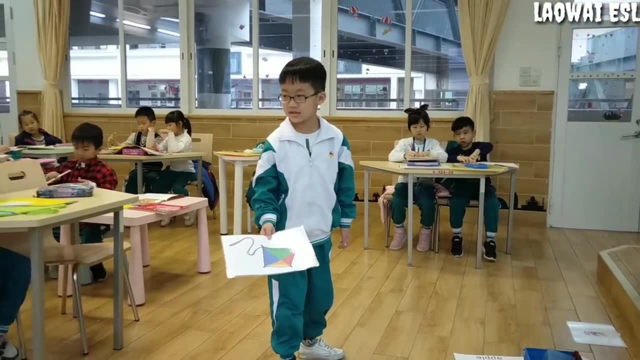 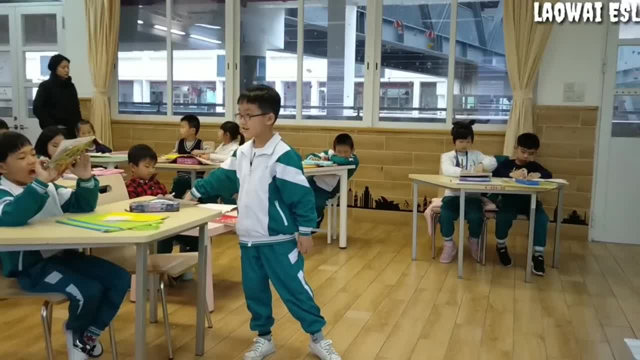 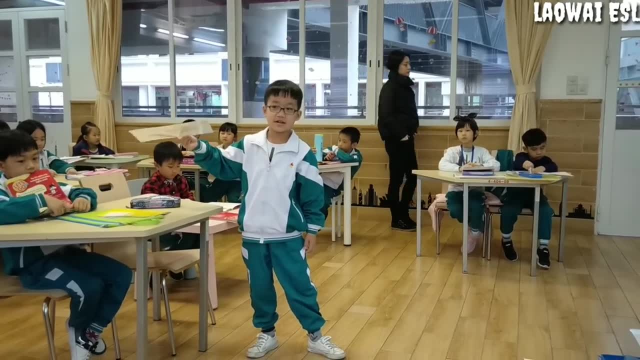 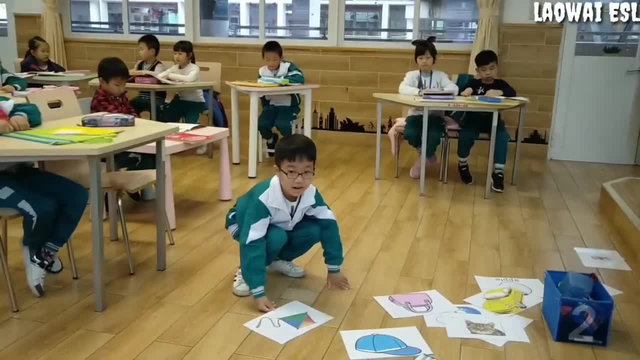 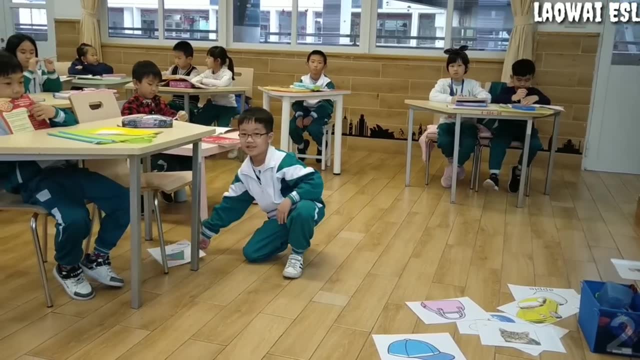 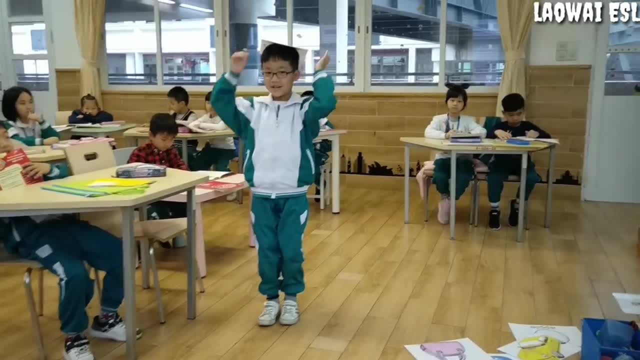 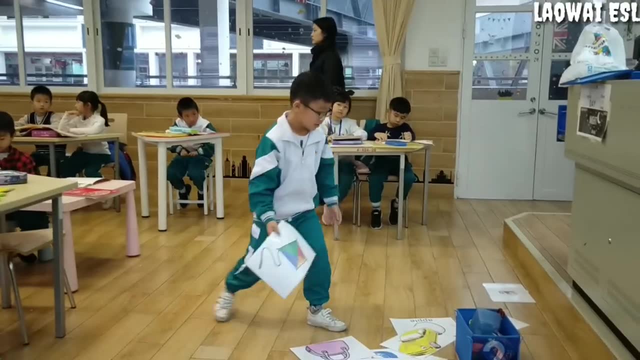 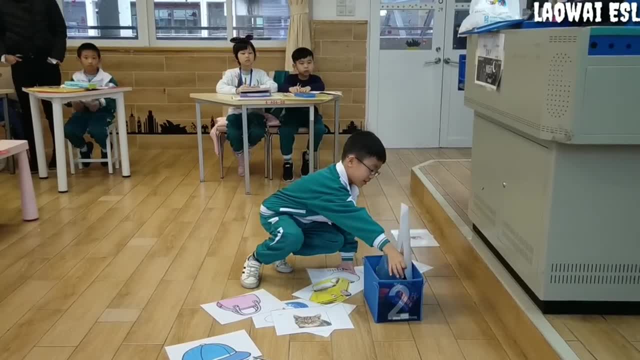 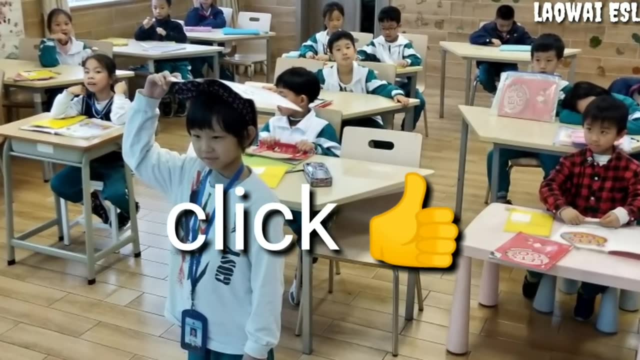 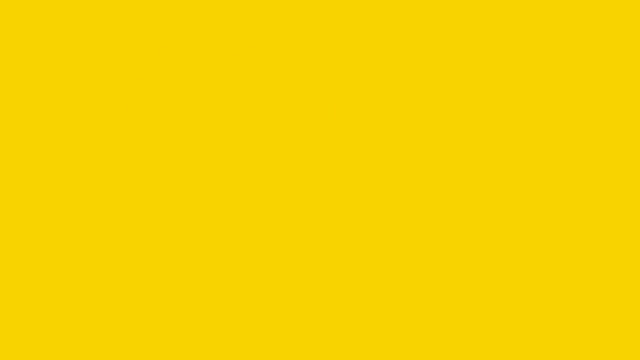 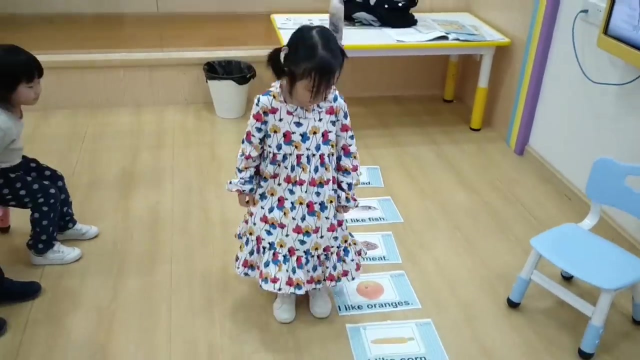 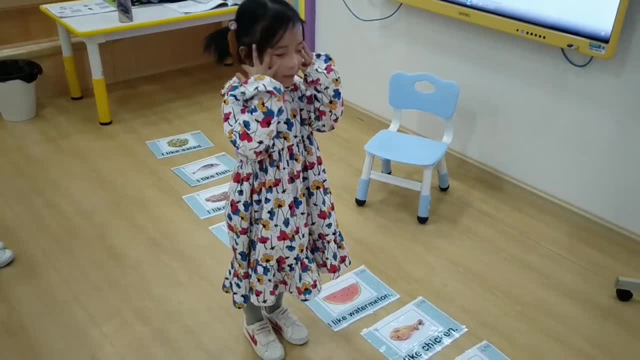 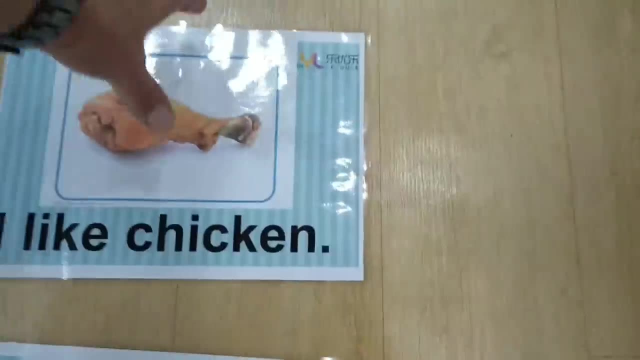 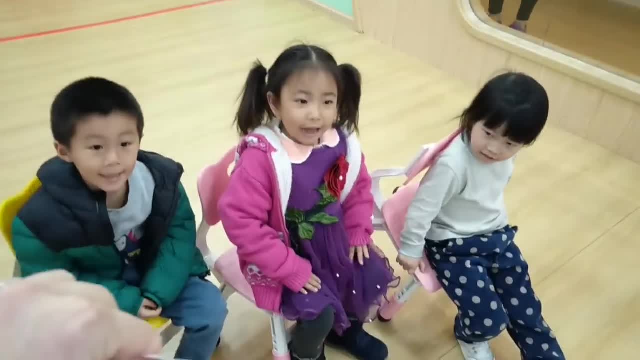 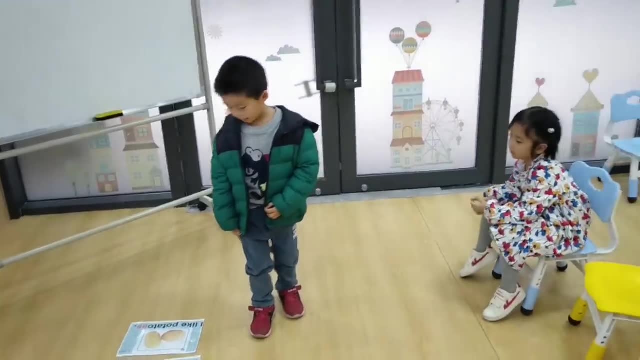 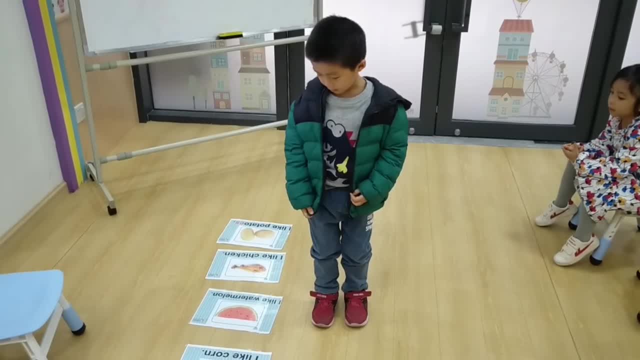 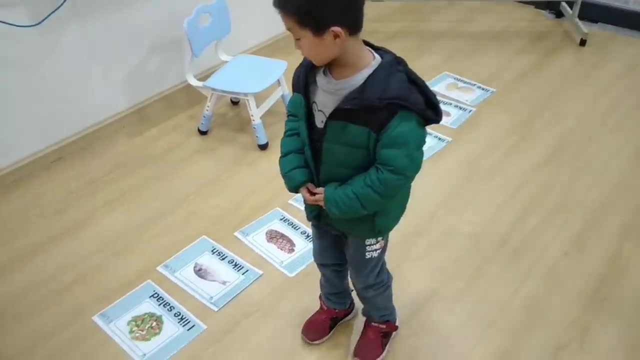 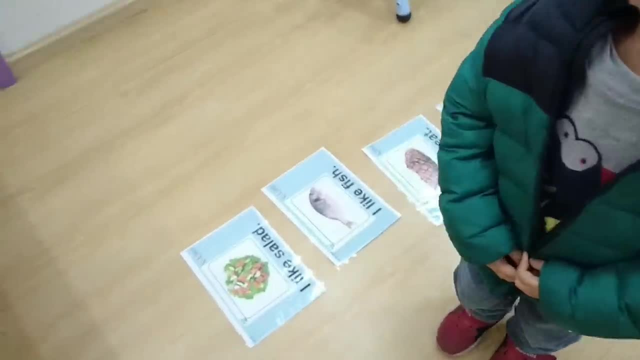 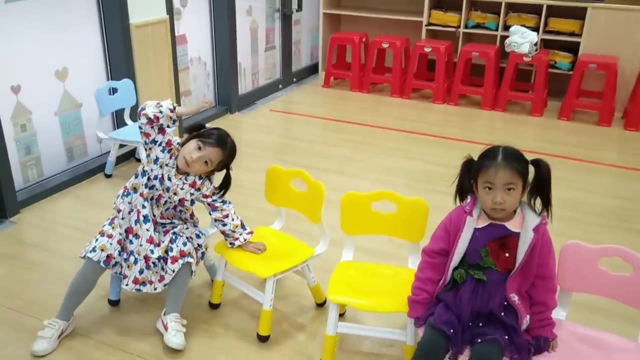 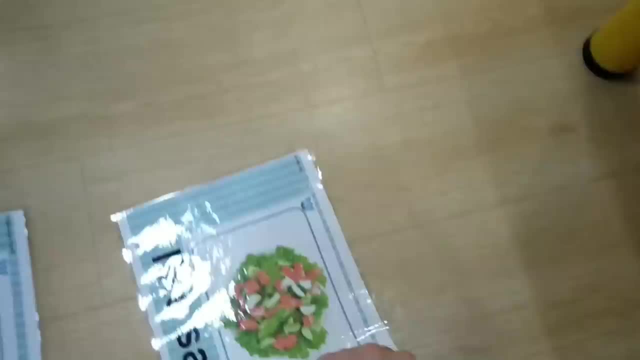 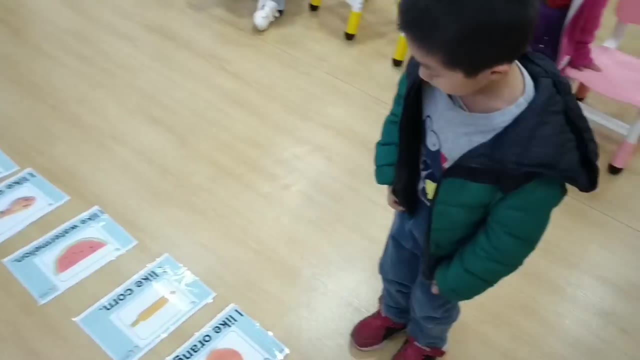 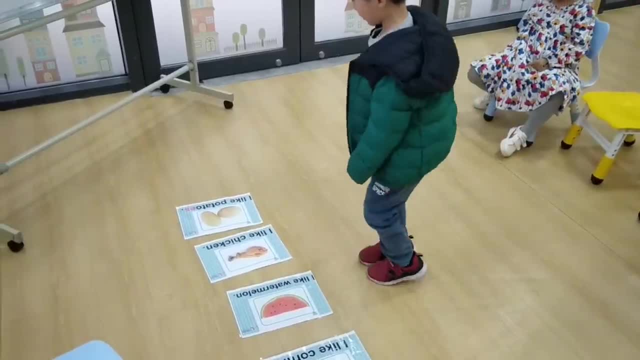 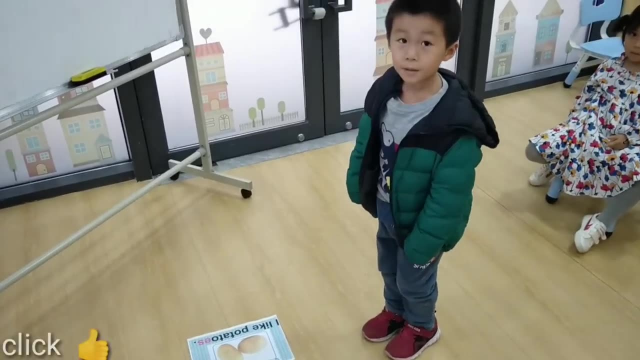 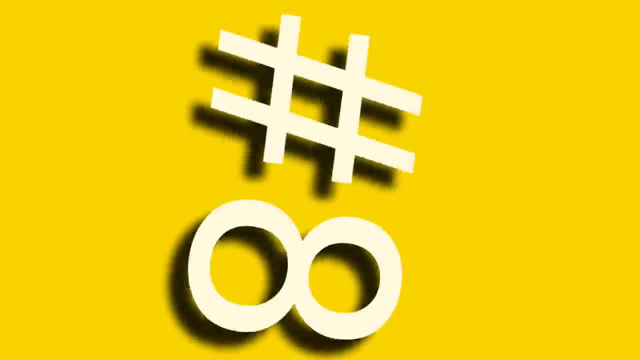 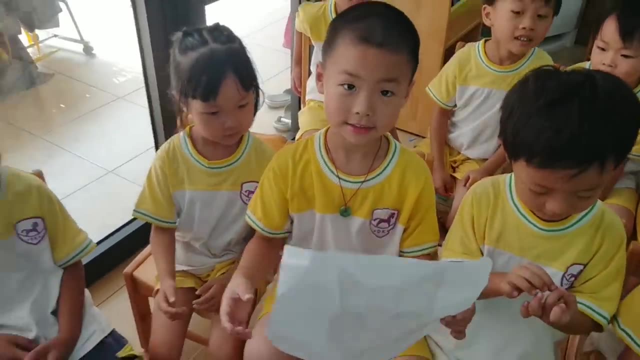 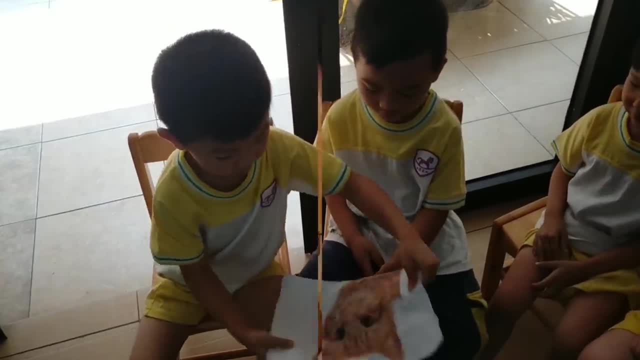 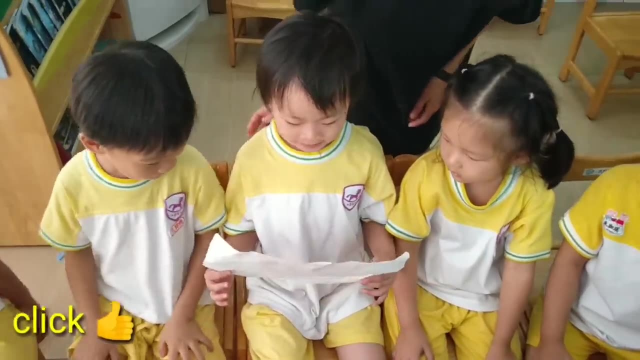 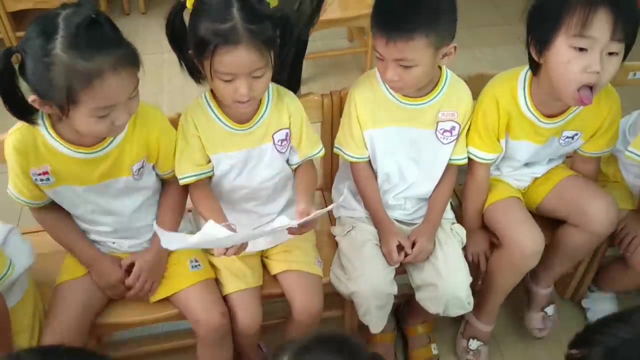 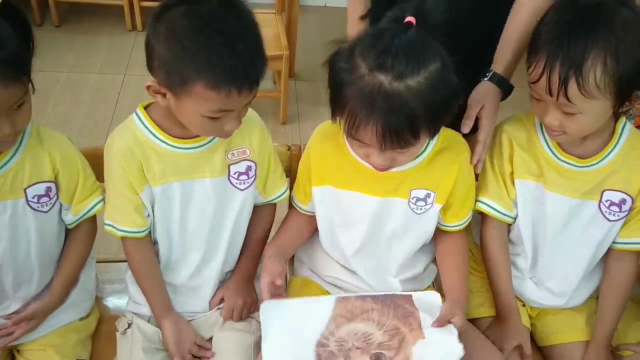 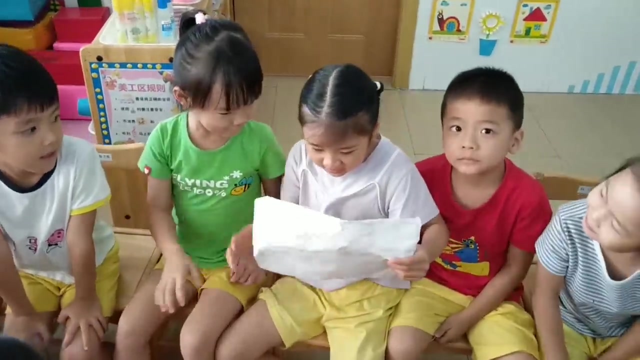 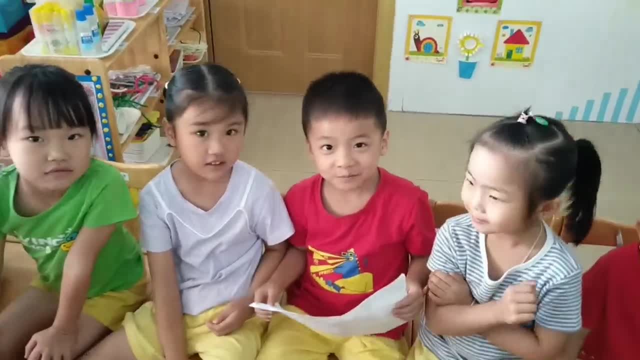 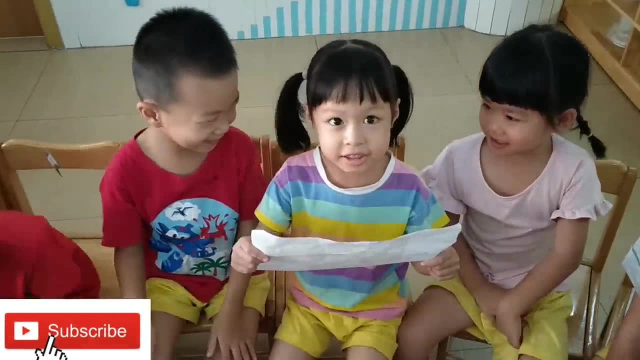 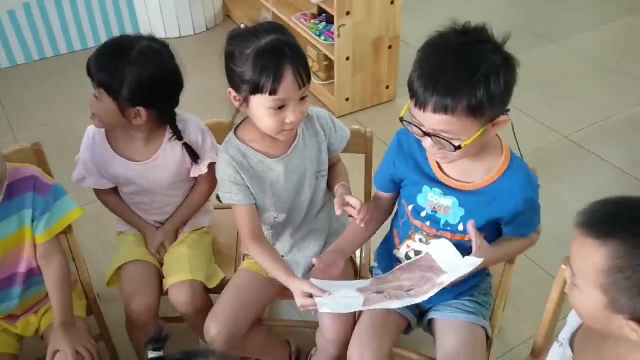 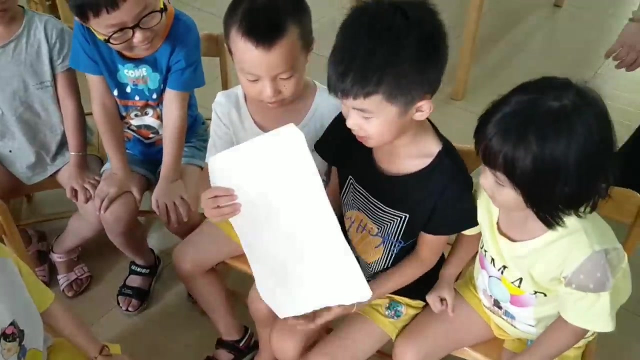 Very good. Come, Come Cat. Well done, excellent, Your neighbor, Thank you Very good. Jump Very good, Excellent Cat. Well done Very good. come on next one. Good job, Well done, Very good. let's give it to you and say cat. 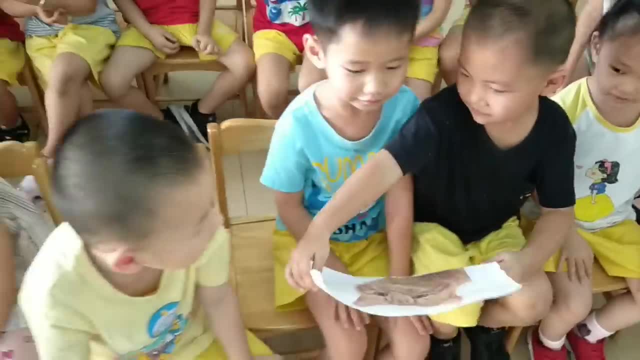 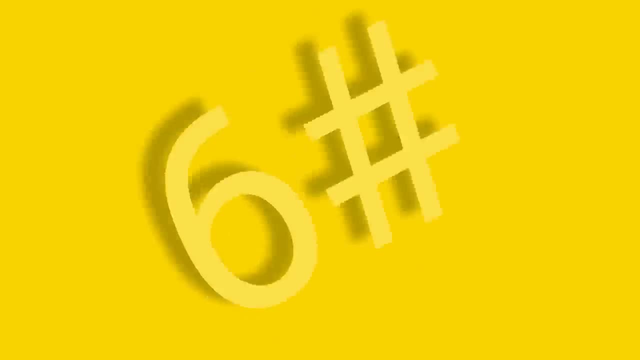 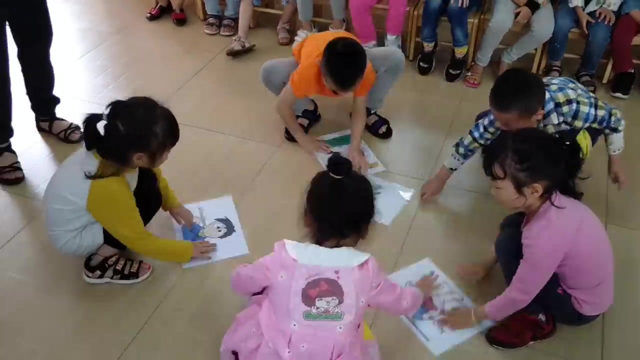 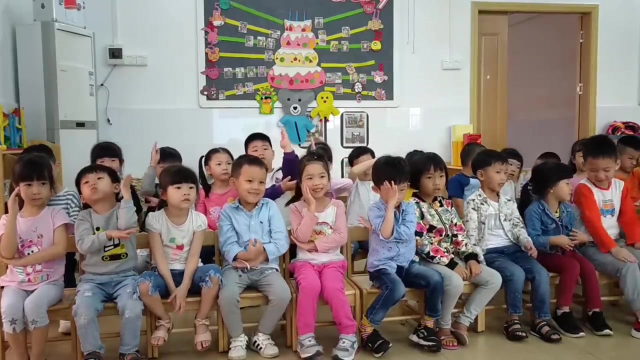 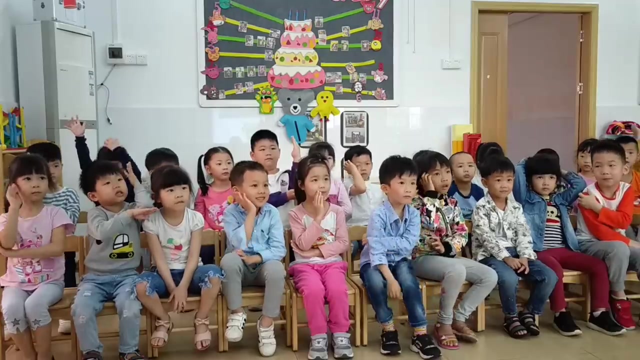 Very good. Okay, Cat, Very good, If you guys want to play the game, show your hands From down. only show your hands, Cat. Now you stand up, come here, Stand up, come here. All right, stand up, come here. 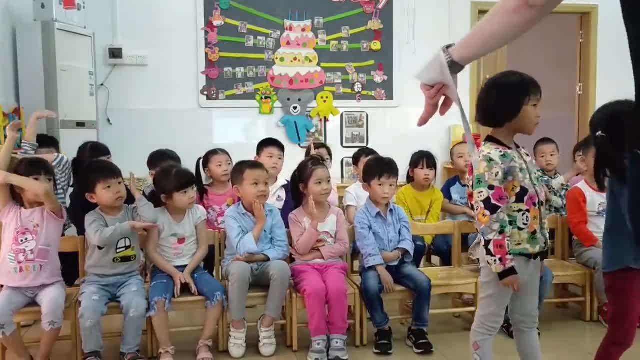 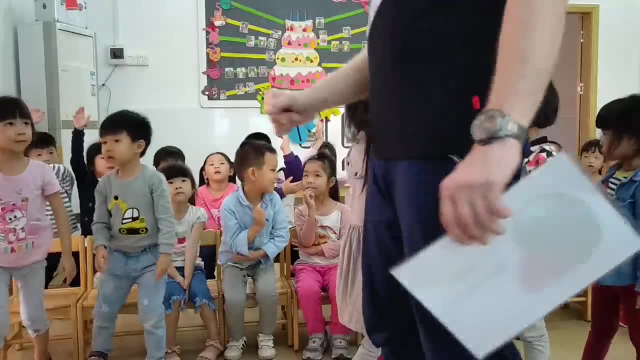 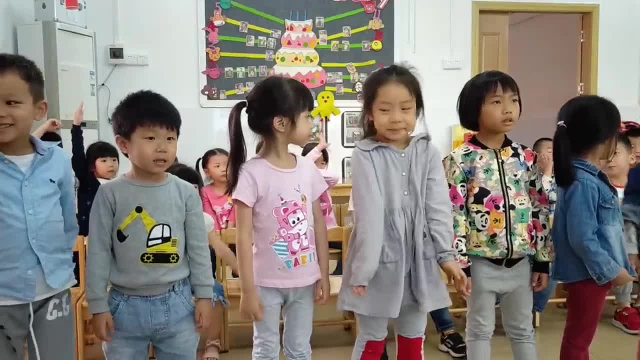 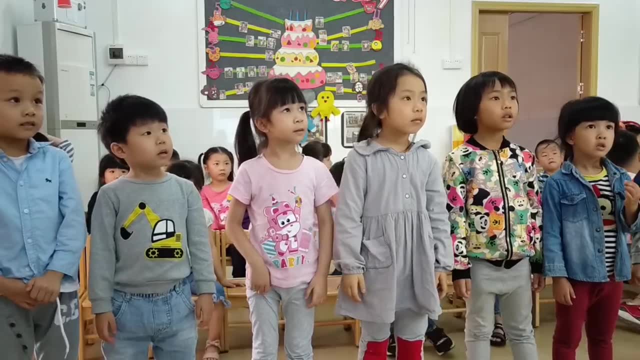 All right, come here. Okay, stand up. Well done, You like it. you did not pass this. Okay, now, guys, if I put the flash card here, you should jump and say: what's the matter? Okay, What's the matter. 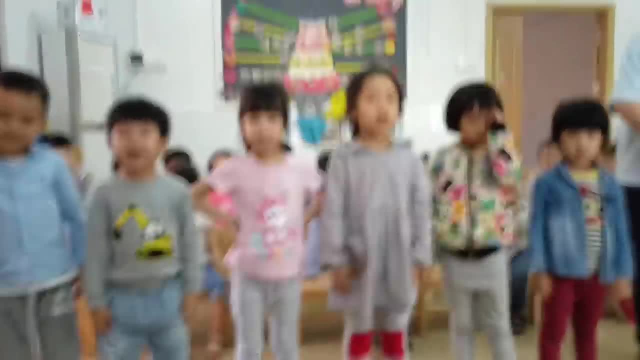 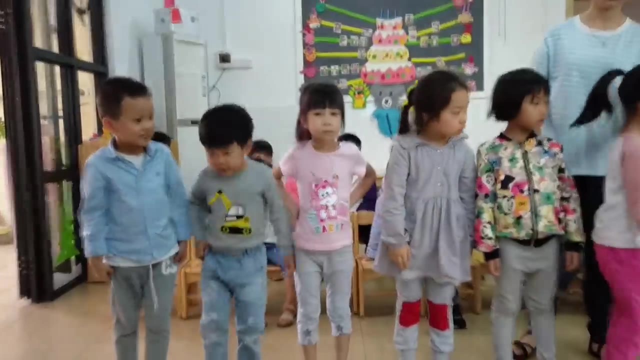 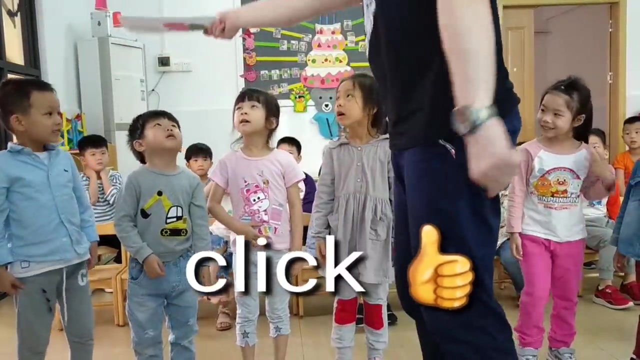 I don't understand. okay, What's the matter? Well done, let's do that again. Come on, guys Ready. All right, One, two, three, let's go, man. What's the matter? What's the matter, Okay? 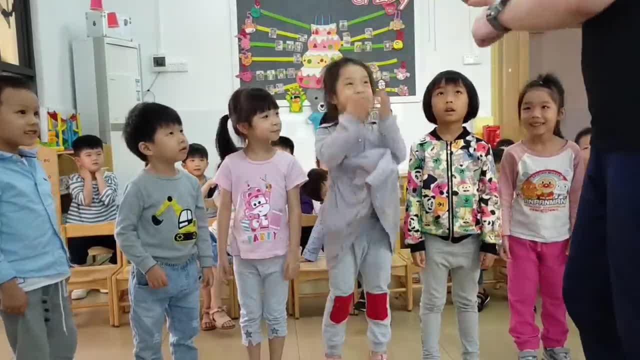 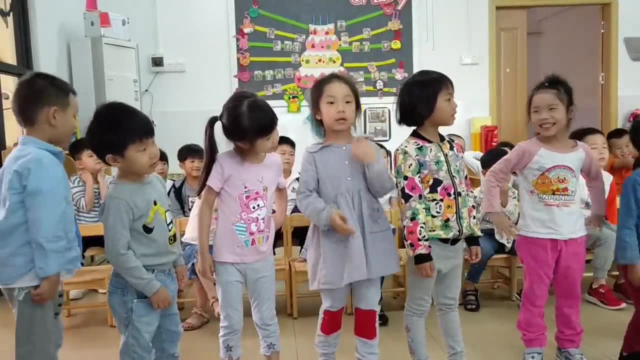 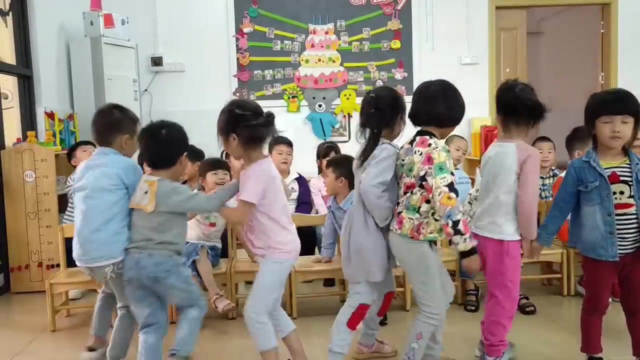 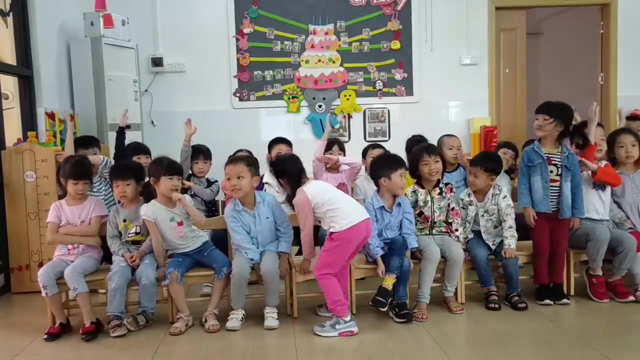 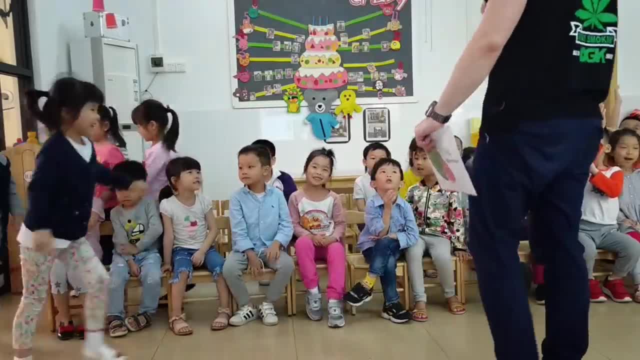 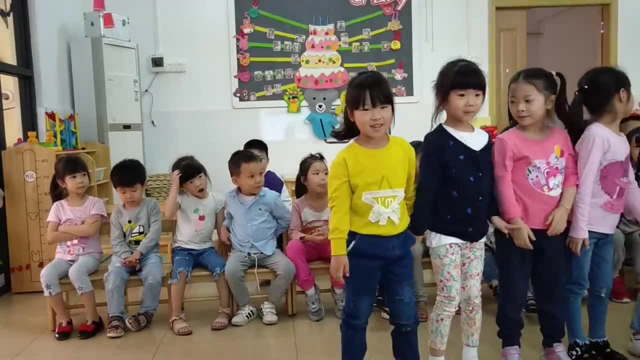 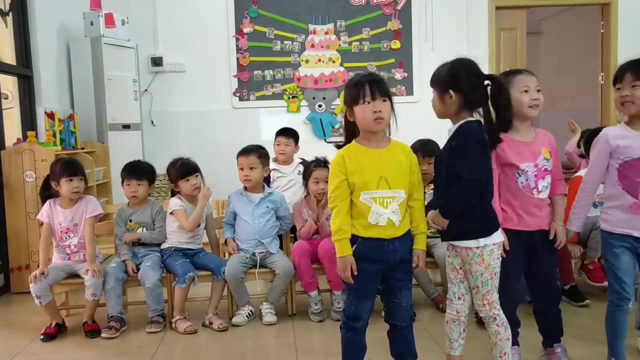 Okay, Okay, Good job, Welcome. What's we playing here, marktlah, American cremate we made. Get out of here, guys get out. Okay, stand up, guys. Make the line over here, Alright. First of all, everybody look at me and say watermelon. 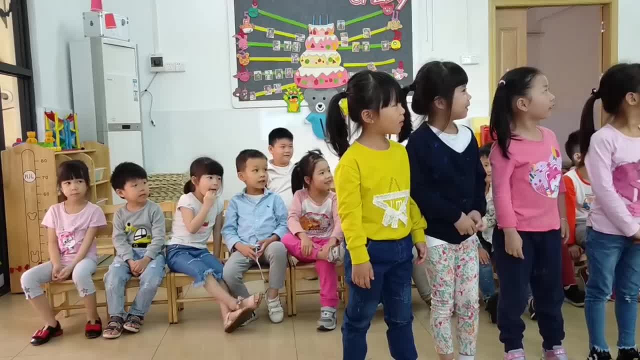 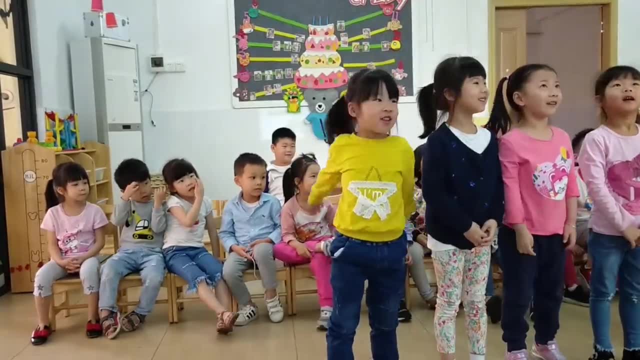 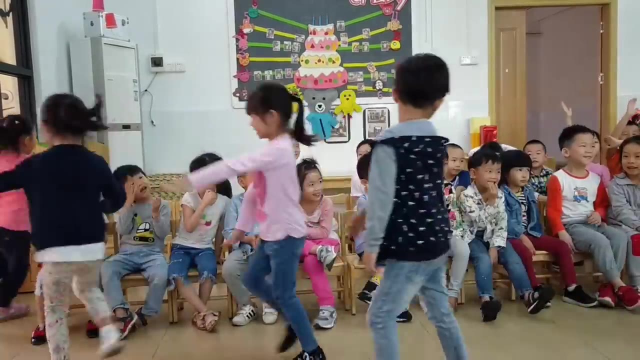 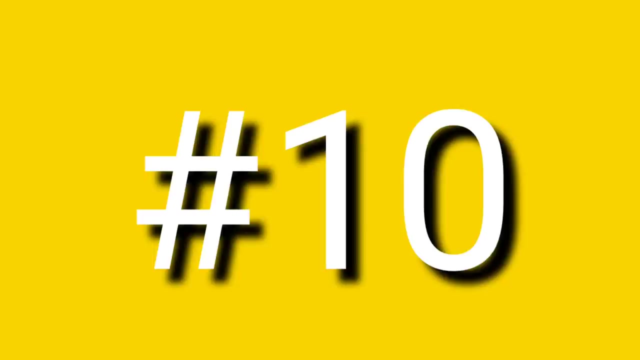 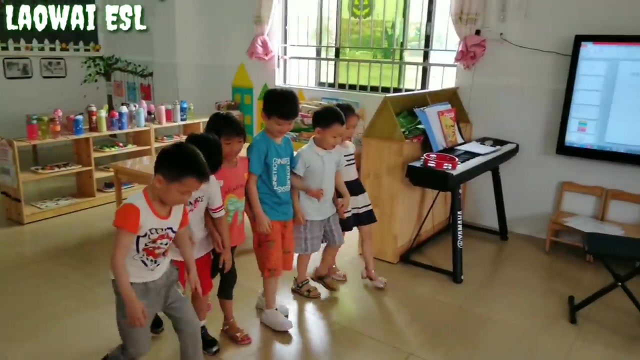 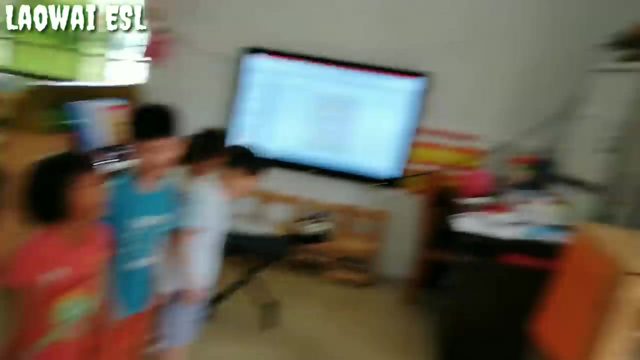 Watermelon. One, two, three, let's go. Watermelon, Wonderful, Very good Watermelon, Great job. Watermelon, All the way, Watermelon, Watermelon, Watermelon screams. What are they saying 4 o'clock? 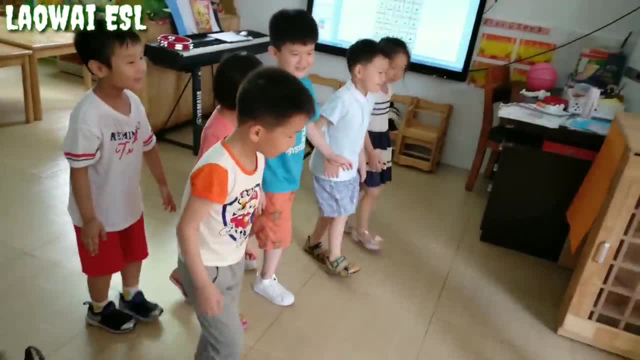 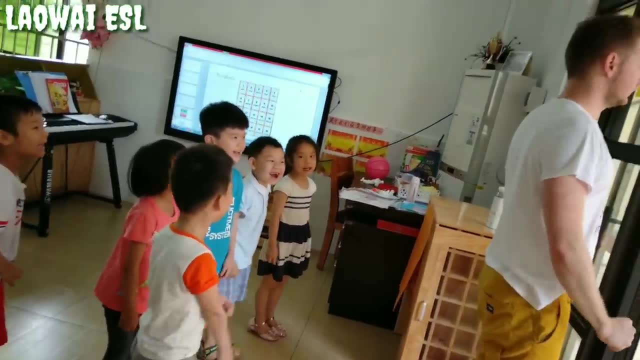 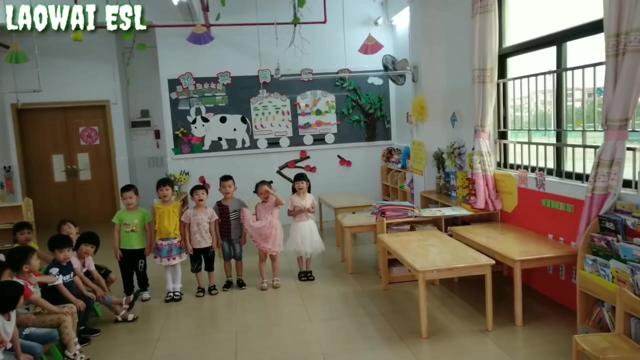 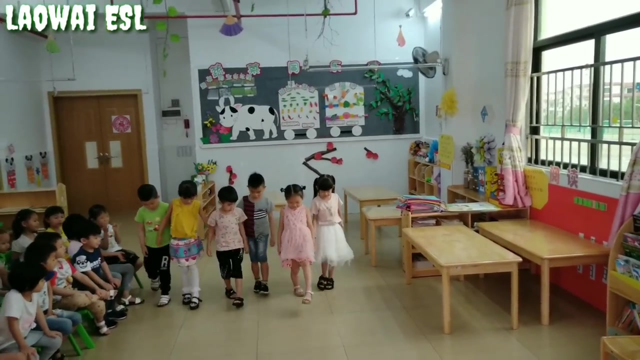 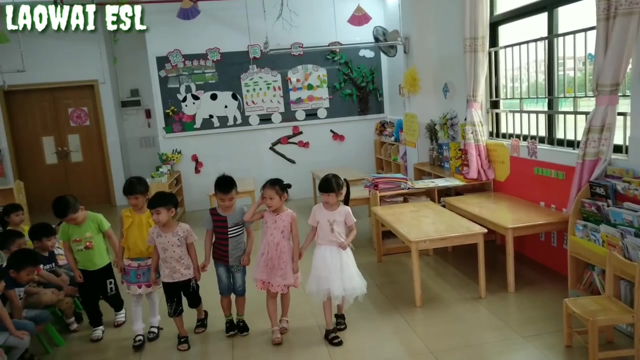 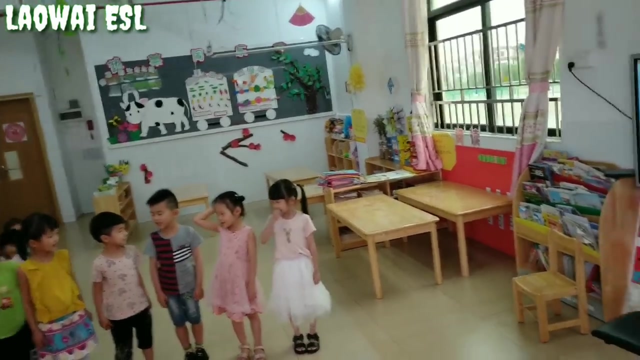 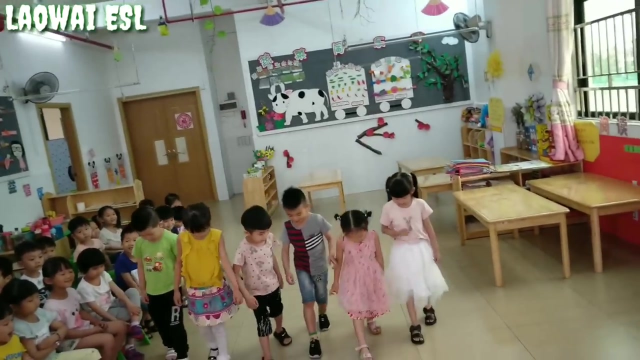